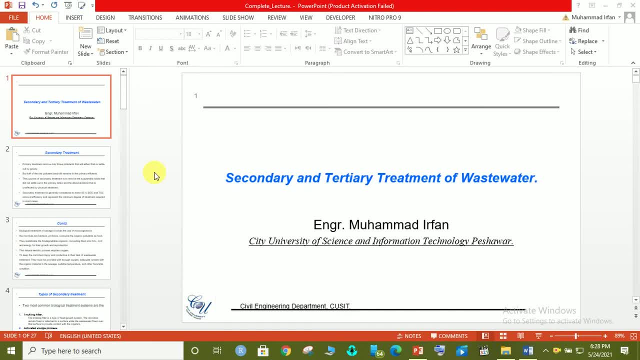 Today we will start our new lecture. The title is Secondary and Tertiary Treatment of Wastewater. From the couple of weeks we started a new series of lectures on how to treat a wastewater- from domestic wastewater, industrial wastewater and other types of wastewater. 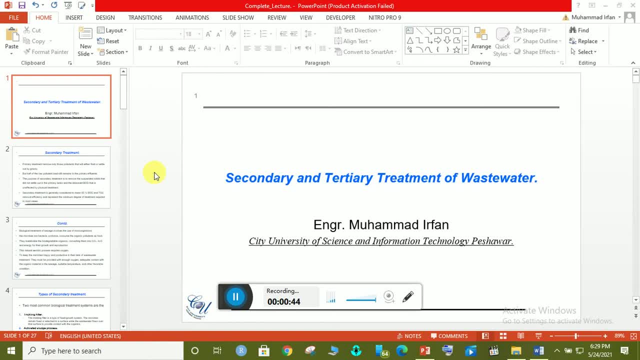 To continue this topic, we start from the beginning, which is the preliminary sedimentation process, After that, primary sedimentation and the different steps that are involved, and the primary sedimentations are coagulation, flocculation, skimming tank, primary sedimentation tank. 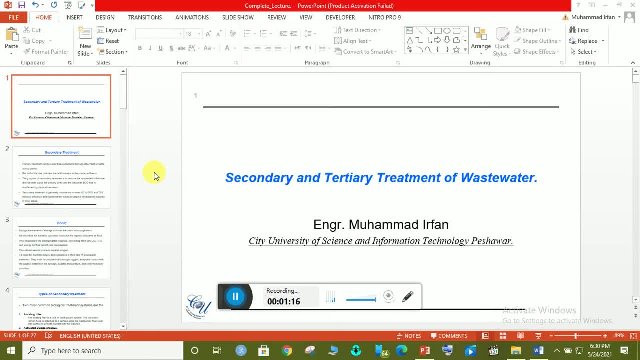 etc. During the primary sedimentation We basically start the primary sedimentation process. We basically treat the wastewater by screening, by grid removal, and after that the wastewater still contains some suspended organic solids that can be removed by the plant sedimentation, which is called the primary clarifier. 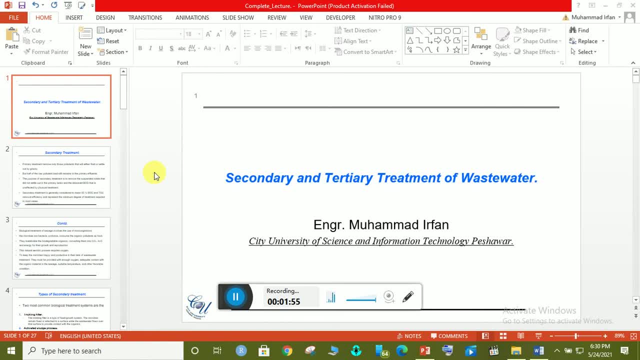 But obviously The, The wastewater are not completely cleaned. So the primary treatment process: remove only those pollutants that will either float or settle out by the gravity, But most of the raw pollutant, most of the pollutant load still remains and that of the 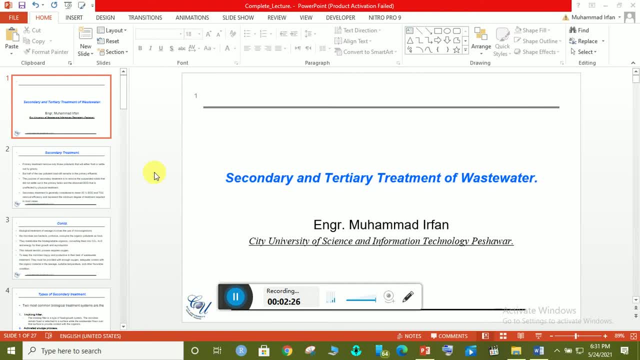 wastewater And the form of suspended solids, and most of these suspended solids did not settle down under gravity, Which is obviously some dissolved organic solids. The dissolved organic solids is also called the BOD- biochemical oxygen demand. The secondary treatment is generally Considered to remove the BOD and total suspended solids from the effluents. 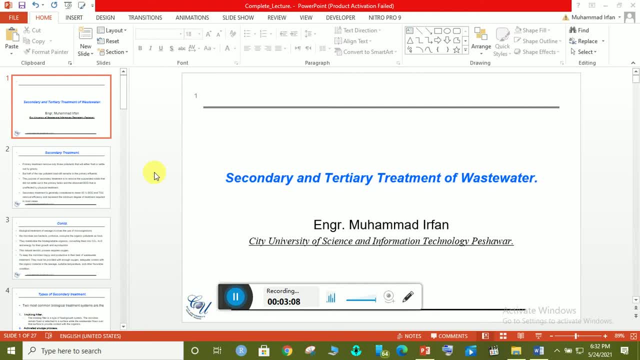 Effluents means that the wastewater coming from the primary treatment, we clean the dead effluents from the primary treatment of about 85 percent. Cleaning means We clean the effluents, We clean the effluents, We clean the effluents. 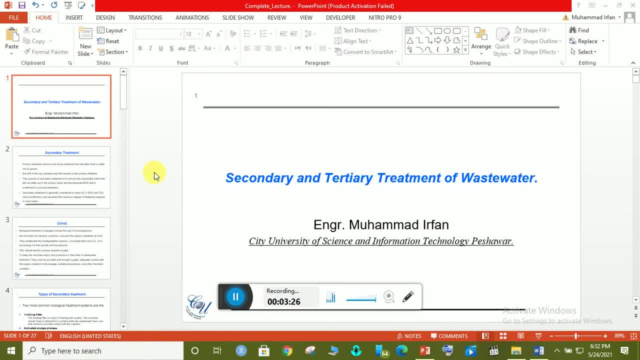 The secondary cleaning means to remove the suspended BOD and total suspended solids. So let's start the secondary treatment. What are the dip? What are the basic concept of the secondary treatment? How to treat the secondary treatments of a secondary. How to pause the wastewater from the secondary treatment. 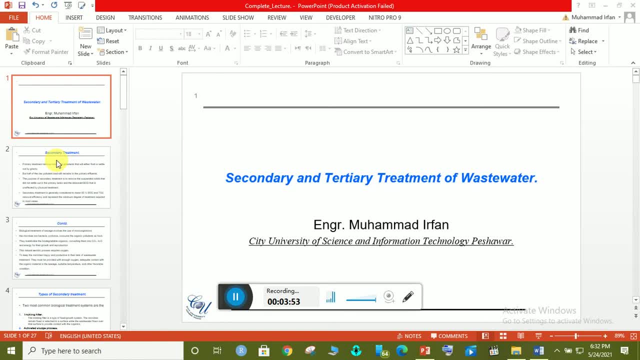 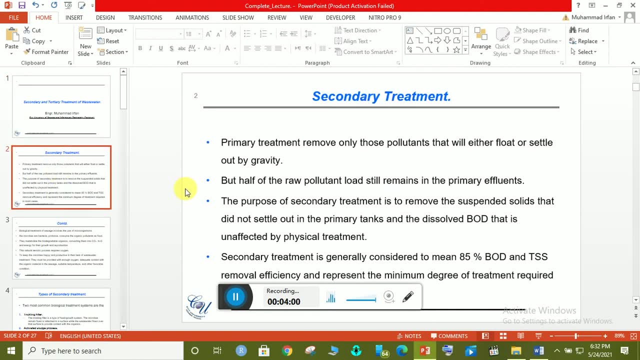 What are the different types of secondaryUs And their property types? So let's start the secondary treatment treatment and their tertiary treatment. what we can do in our in a tertiary treatment, so primary treatment- remove only those pollutants there that will either float or settle out by the 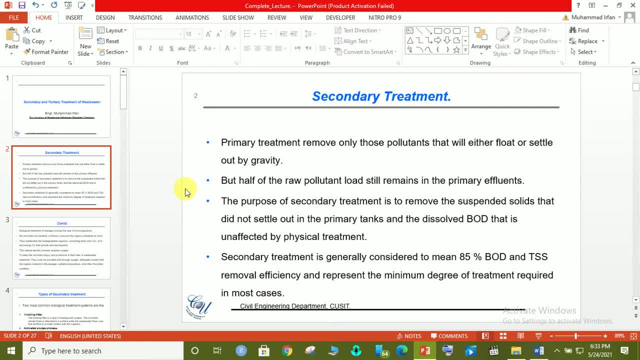 gravity, jo, which the topics: primary treatment, the primary treatment by you under gravity, to have a settle, or Jata has a term at love Nietzsche bed Jata, yeah, surface pair floating career today, yes, suspended form. may hotel to vote to primary treatment major have a multiple process, a pass, okay, we'll. sorry cheese's, you have a tonic al Jati has. 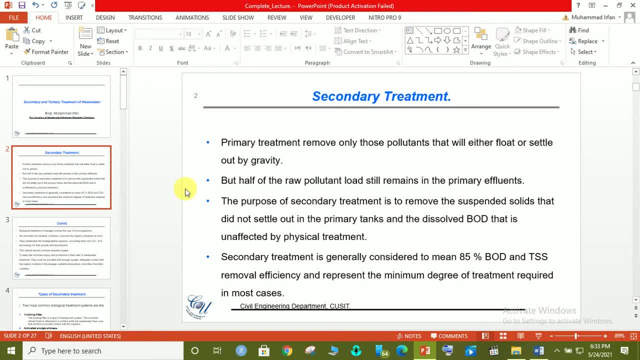 ponies waste water, say, but half of the raw pollutant load still remains in the primary influence, like in pill B. to have a up deck second hand cage of Amara mama pass your wastewater hair was still to have all this. got girls, I have a turbid. 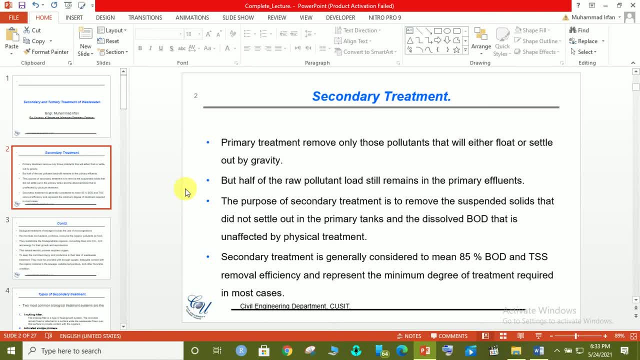 hair this come up of? yeah, I gave a smell which, no, could you have what she's, a mood with her. so the purpose of the secondary treatment as to remove the suspended solid- they did not settle out- and the primary trains and tanks and dissolved beauty that are unaffected by the physical treatment. so secondary: 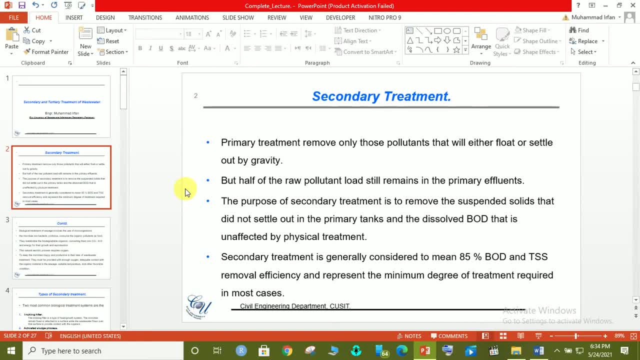 treatment. my home, you cut ahead K Joe, this is Joe. particles hair or under gravity. you have a settle new Jata or, yeah, dissolved solids hair, dissolved organic solids. hey, just come, beauty, be kept a hand. whoa, you have under gravity. you have a Nietzsche naive, a Jati. to this, to this kill, you have a secondary process to have. 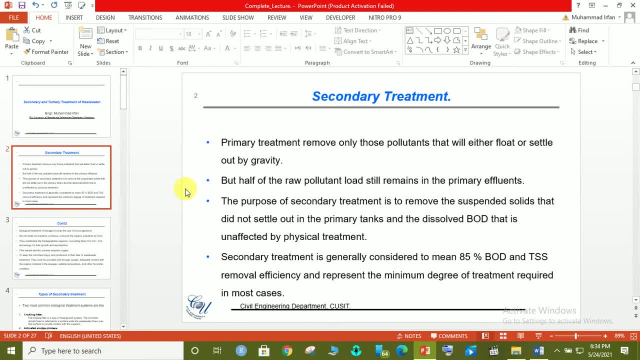 occur later. so yeah, a question hacky. suppose Amara pass water hair or is may, which is you have or dissolve over here. suppose apnea chini to have a water may dissolve key here to kiss the round. push Cheney, Minnesota yoga. we have a lot of offers and a very interesting method of 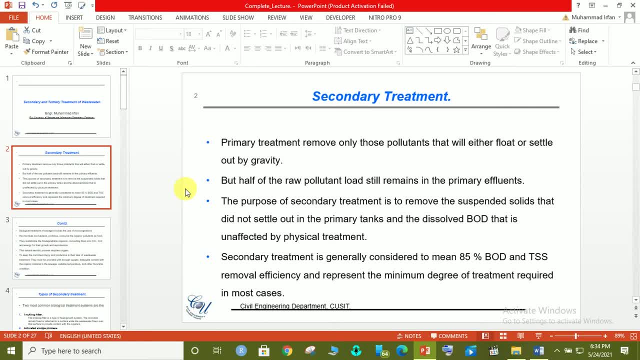 all the processes that we have to go through here about sugar, we will also go through the process of the process. we should know this is very important because as we go through so we know that there are some organic solids that we will the water, and also most of the water that we have is a lost one. so 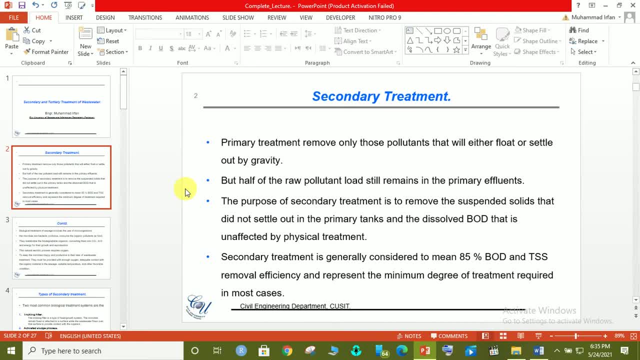 now we are doing the same thing, so the process will not be the same at all. we also know that the water, what we also know, and we are going to use it for a specific purpose, and that we are going to use it for the specific purpose that was. 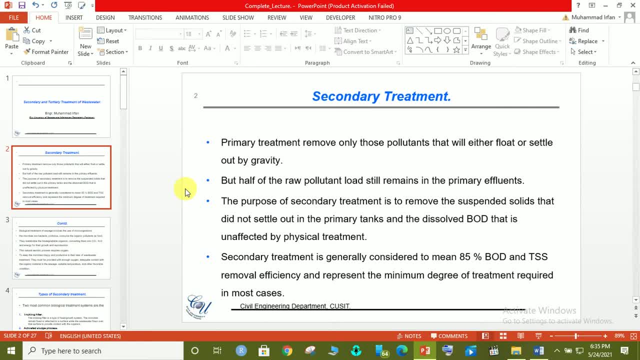 We take gravels of a specific size and the water that comes from the primary treatment in which these not-settlable solids or dissolved BOD are present. then we pass that water through the filter media. In this process, the bacteria start generating in the filter media. 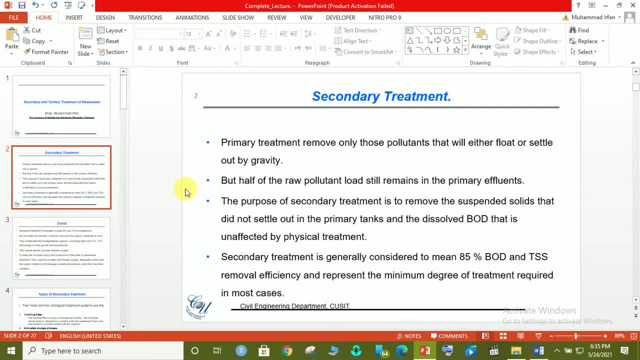 and different kinds of microorganisms make the dissolved BOD their food and convert that dissolved BOD into undissolved BOD. We know that undissolved BOD that is when it is converted into undissolved particles. then the undissolved BOD easily sits down. 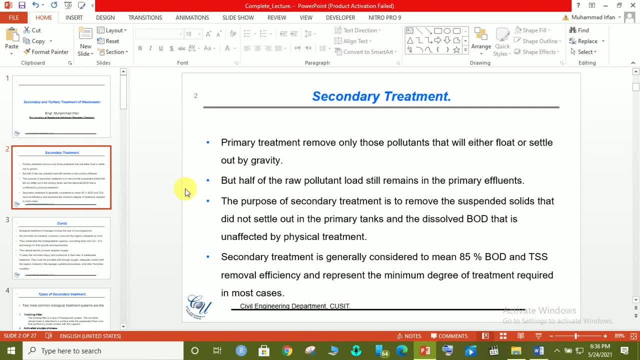 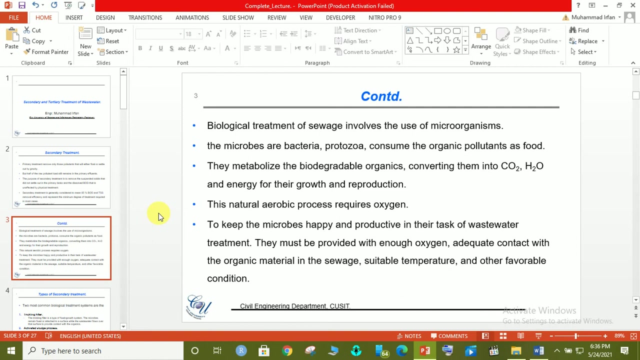 and we remove it in the secondary sedimentation tank in the second process. So this is the whole process. Suppose 85% of BOD, or total suspended solids, is removed from the water through secondary treatment. Biological treatment of sewage involves the use of microorganisms. 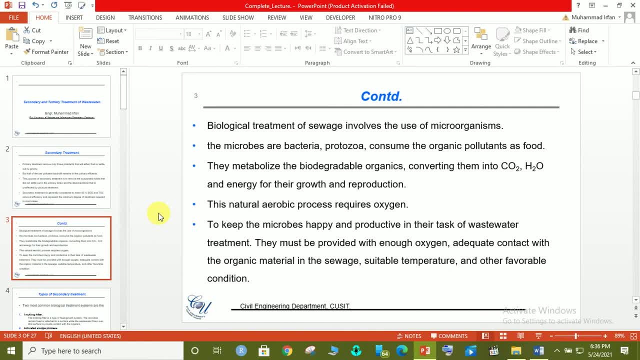 I have told you that we use microorganisms for biological treatment. Secondary treatment is also called biological treatment because this process is done by biological means, by the use of bacteria, by the use of microorganisms. The macros or bacteria are protozoa or bacteria. 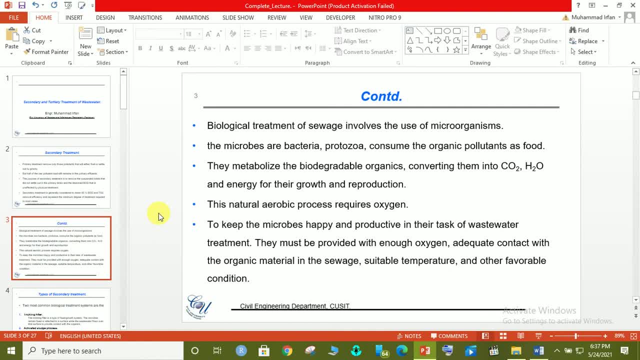 And those are the organisms. the organic pollutants are metabolized or utilized as a food, And that dissolved organic BOD is converted into biodegradable organics. It is converted into carbon dioxide, water and energy. This natural aerobic process requires oxygen. 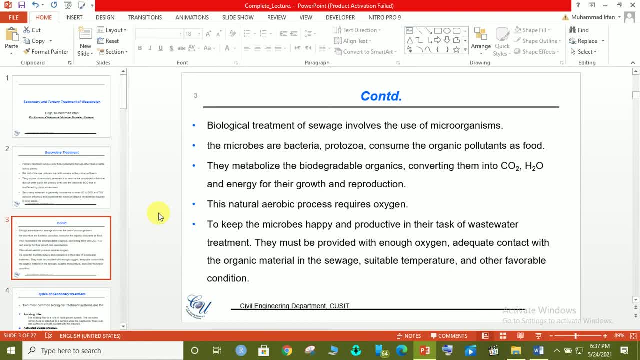 So the way you know that bacteria, in the presence of oxygen, need oxygen for the reaction of their metabolism or food. So when they use oxygen there is a lack of dissolved oxygen in that water. So when there is a lack of dissolved oxygen, 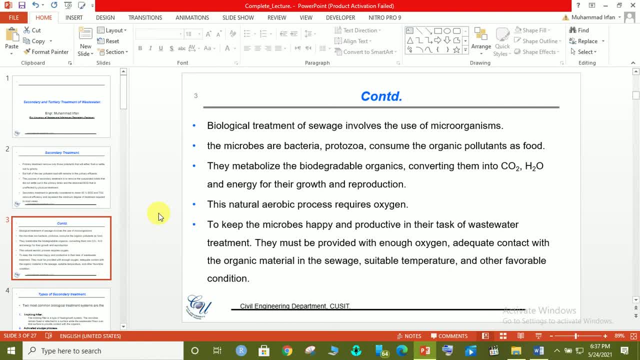 the oxygen demand in that water increases, The BOD level increases. So to keep the microbes happy and productive in their task of wastewater treatment, they must be provided with enough oxygen, adequate contact with the organic material in the sewage, suitable temperature and other favorable conditions. 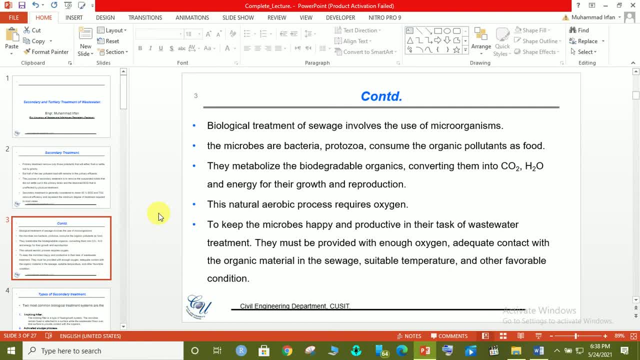 If you want to eliminate your secondary process, that is, the dissolved particles, then you have to keep your microbes happy. That means if it needs oxygen, then you have to provide oxygen through the aeration process. Aeration means that you have to provide oxygen manually. 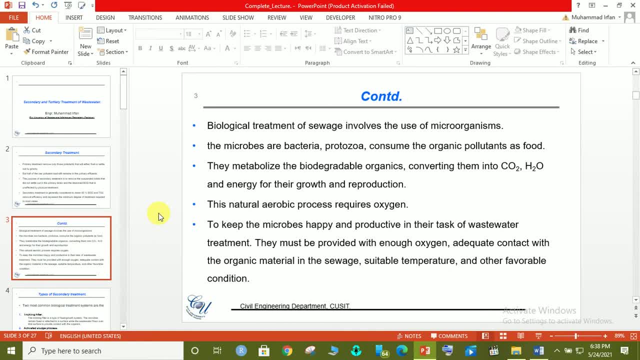 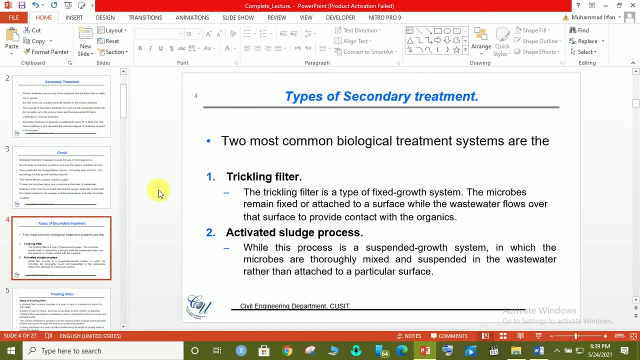 or a diffuser is installed at the bed, It provides enough oxygen. In this way. if organic materials are available in large quantities, then those microbes are happy And the reaction of their metabolism starts And it gets faster. In this way there are two types of secondary treatment. 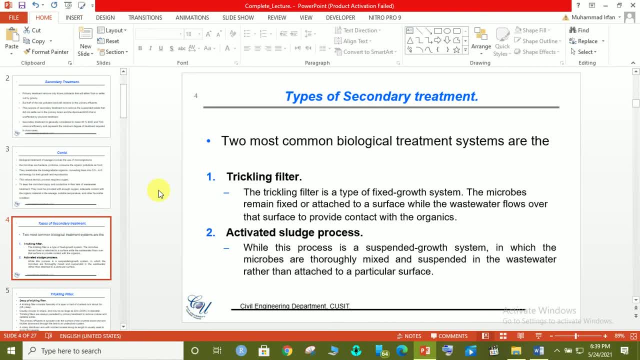 One is called trickling filter and the other is called activated sludge process. So the trickling filter is a type of fixed growth system. There are two things in it. One is a suspended growth system and the other is one is. 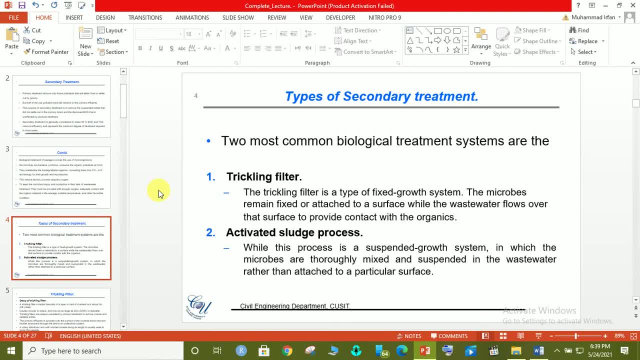 suspended growth system. So what is the difference between these two? The microbes remain fixed or attached to the surface, while the waste water flow over the surface to provide contact with the organics. I will explain it to you easily. Suppose we have a filter. 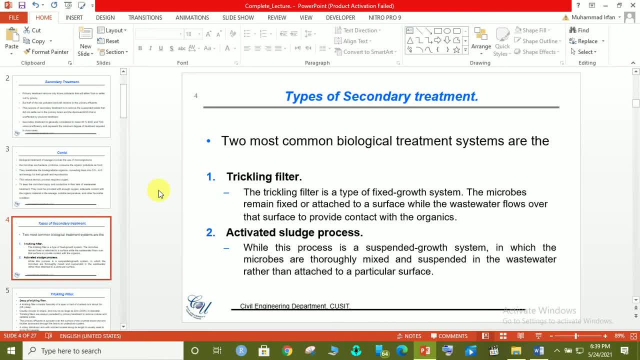 Filter means that we have some big stones from which we have made a filter media. It is of a special width And we pass the same filter media, which is a fixed width and a fixed surface through which we pass our primary effluent. 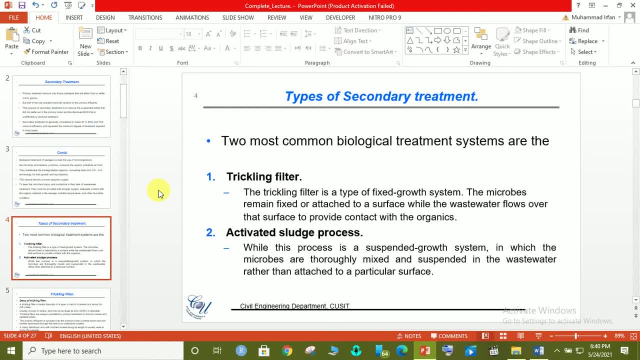 that is, the waste water that comes from the primary sedimentation process through that filter. So the microorganisms present in the filter start their work, The metabolism reaction starts And in this way the dissolved particles are converted into the undissolved form. 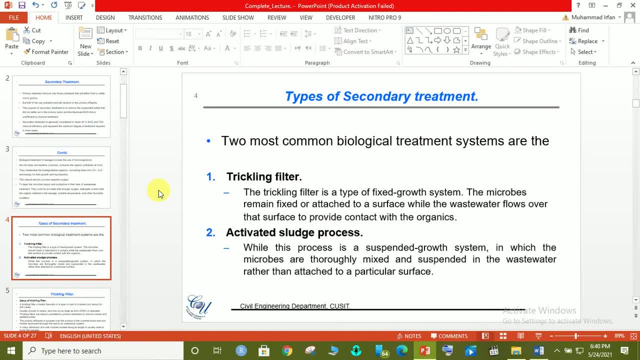 In this way, there is an activated sludge process. So what we do in this is: the surface is not fixed. We have an effluent from the primary. that is, the effluent that comes from the primary, the waste water that comes. 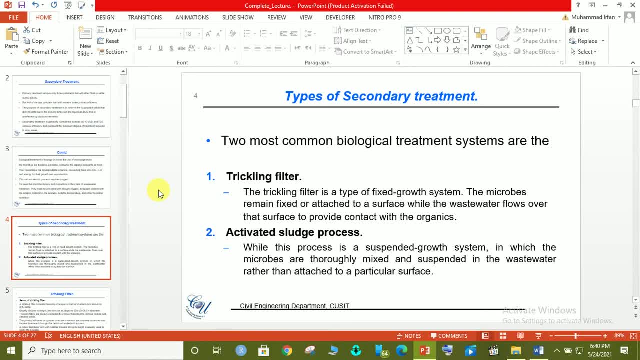 we mix that waste water with the microorganism, We make a slurry And in that whole media the microorganism starts its work And in that the metabolism reaction starts And the dissolved particles are converted into the undissolved form. 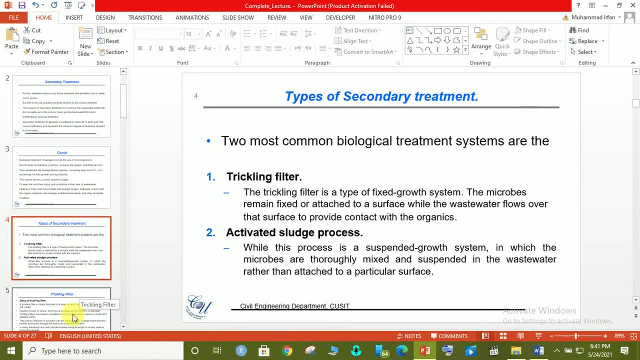 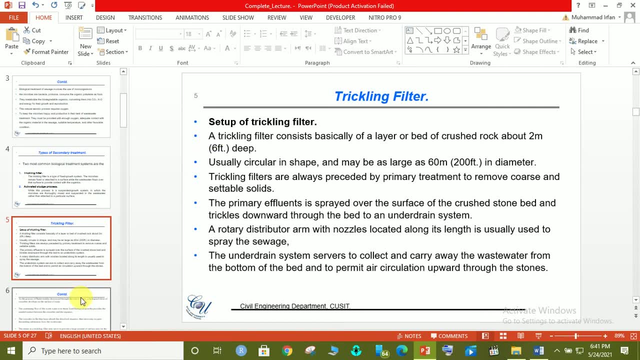 This is what we call the activated sludge process, And we will study this in detail, InshaAllah. So the first one is the trickling filter. I have given a link to its video. You can see that too, But its setup is like this. 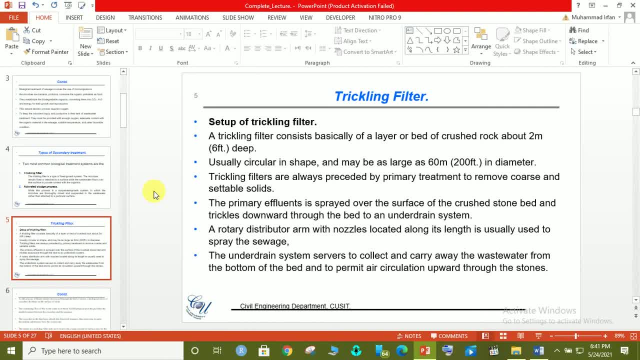 Basically, a layer of crushed stone is about 2 meters or 6 feet deep, Usually circular in shape, Maybe as large as 16 meters or 200 feet in diameter. Trickling filters are always preceded by the primary treatment to remove the coarse and settleable solids. 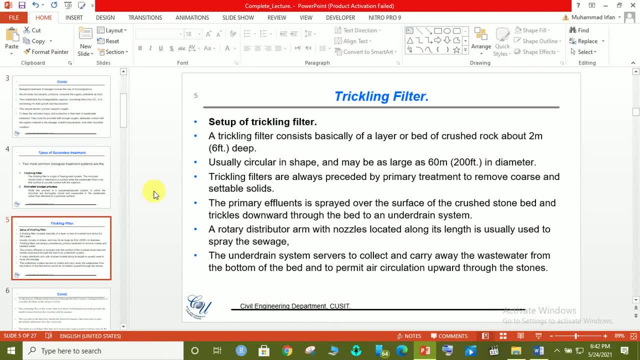 We apply this trickling filter after the primary treatment so that the effluent comes from the primary and passes through the secondary process. The primary effluent is sprayed over the surface of the crushed stone bed and trickles down through the bed to an undrained system. 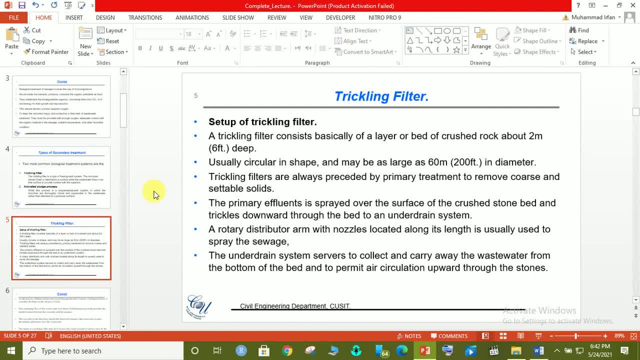 In this way, the undrained system is placed under the rock bed. The undrained system means that the water passes through the stone and accumulates in the undrained system. We spray the primary effluent on the crushed stone bed and it starts to go down for some time. 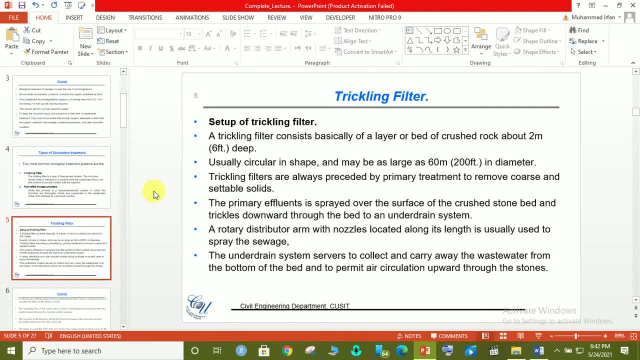 It starts to pass through the filter. When it passes through the filter, we have kept microorganisms in the filter. The microorganism starts its metabolism reaction and in this way the treatment process is completed. The undrained system serves to collect and carry away. 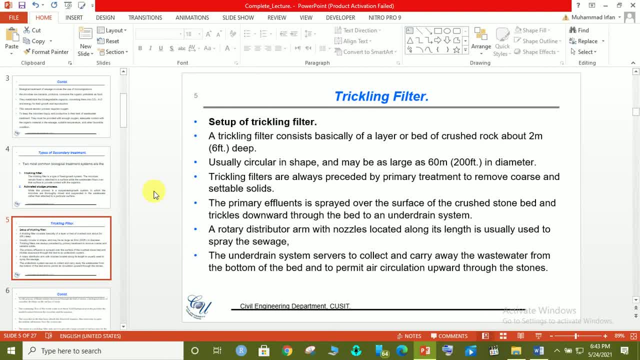 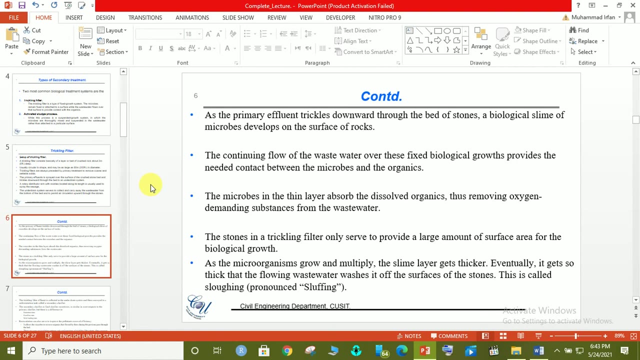 the water from the bottom of the bed and to permit air circulation upward through the stone. These two works are done. First, the waste water is collected through the bottom. Second, the oxygen needed from below is provided for the bacteria As the primary effluent trickles down through the bed of the stone. 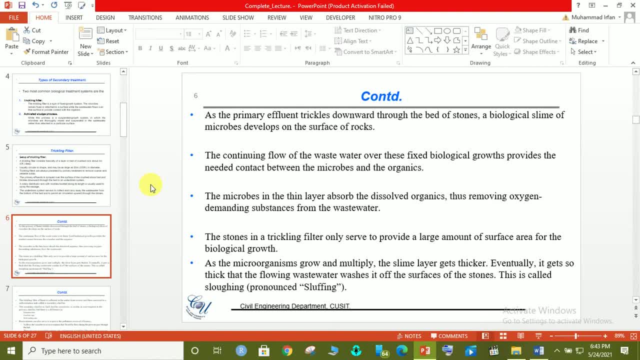 biological slims of microbes develop on the surface of the rock. When the effluent starts to go down through the filter media, a complete biological slim is formed on the surface. The continued flow of the waste water over this fixed biological growth provides the needed contact between the microbes and organisms. 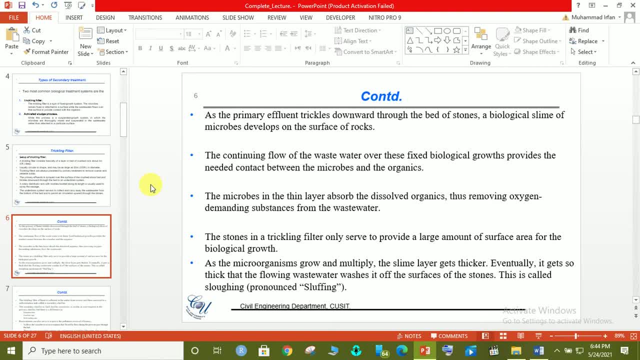 The microbes in the thin layer absorb the dissolved organics, thus removing oxygen-demanding substances from the waste water. This is what I told you. When this layer passes, the microbes absorb the dissolved organics, eat it and convert it into undissolved form. 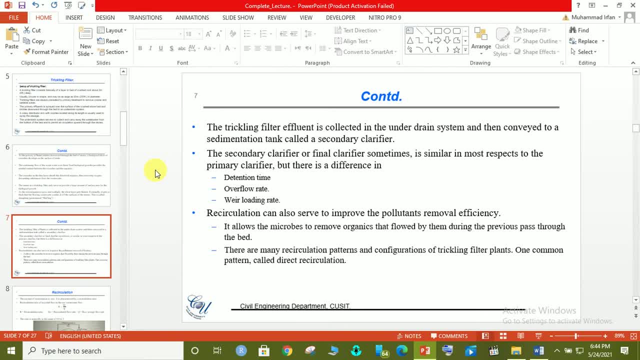 The trickling filter, effluents is collected and the under-drained system which I told you about then. through that under-drained system, when we collect that water, we transfer it to the sedimentation tank. This is called the secondary clarifier. 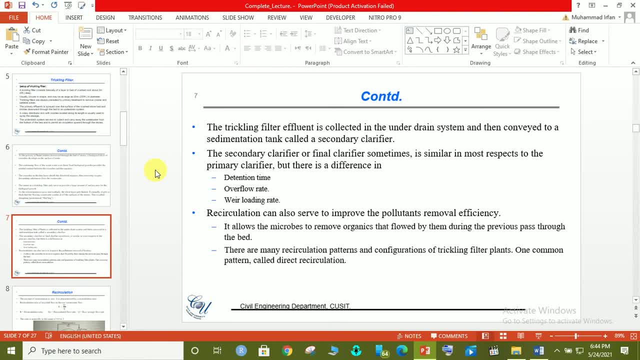 The dissolved particles are converted into the undissolved form by the bacteria. The undissolved particles sit under gravity in the secondary clarifier. The secondary clarifier, or final clarifier, is sometimes similar to the most respect. It is the same thing. 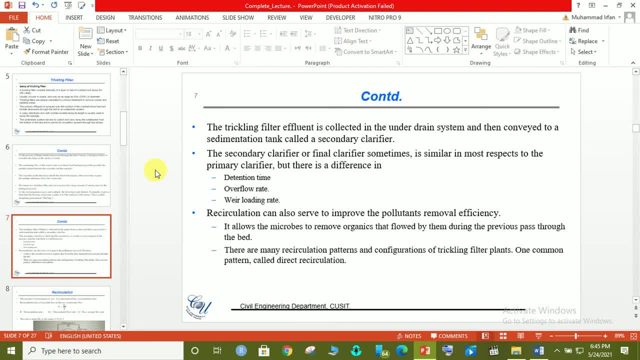 Both are the same tank. One is the primary tank and the other is the secondary clarifier. But the difference is in the retention time. One will be more and the other will be less. There will be a difference in the overflow rate and in the wear loading rate. 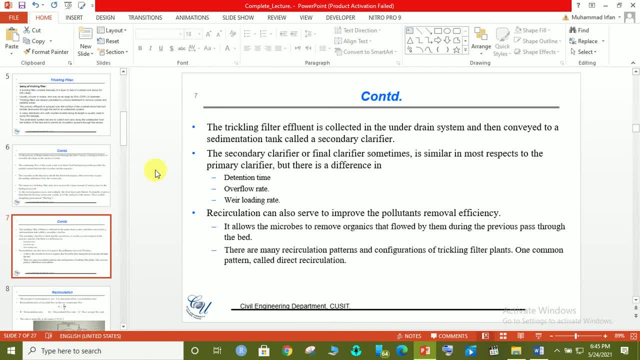 There will be a difference in the values. Recirculation can also serve to improve the pollutants removal efficiency. What does this mean? It means that we process the recirculation. This is the whole topic of recirculation. This means that if you have once passed the primary effluent to the secondary filter, then again we pass a special portion of that effluent to the secondary treatment. In this way, the number of microbes increases. The metabolism rate increases. It allows the microbes to remove organics that flow followed by them during the previous pass through the bed. 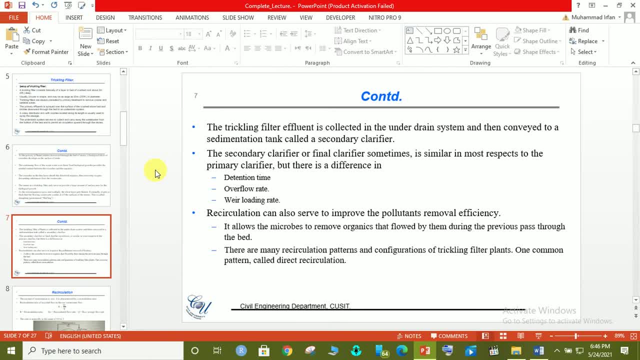 There are many recirculation patterns and configuration of filter plants. One common pattern is called the direct recirculation. There are different types of recirculation. One is called direct circulation. There is a recirculation that happens when the water is in direct circulation. 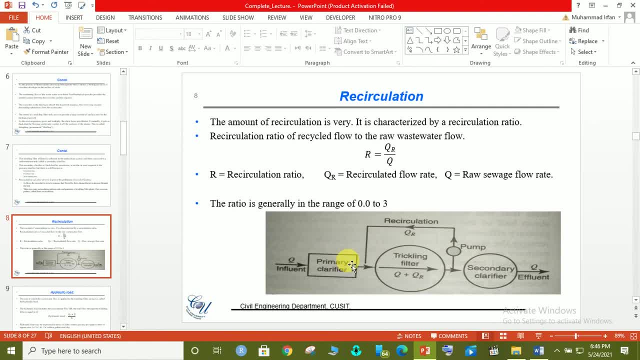 For example, you can see that this is the influent. This is the water that is passed through the primary clarifier. After this, it has been transferred over to the trickling filter. In the trickling filter, the water is transferred from the trickling filter to the water. 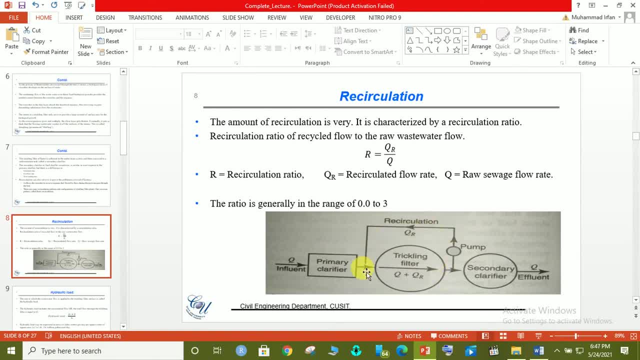 It has to be transported back to the water. If it has dissolved particles, it is converted to suspended water. This is the trickling filter. This is the trickling filter, Another trickling filter. and then the dissolved particles are converted to suspended in the secondary clarifier and they are placed under the gravity. 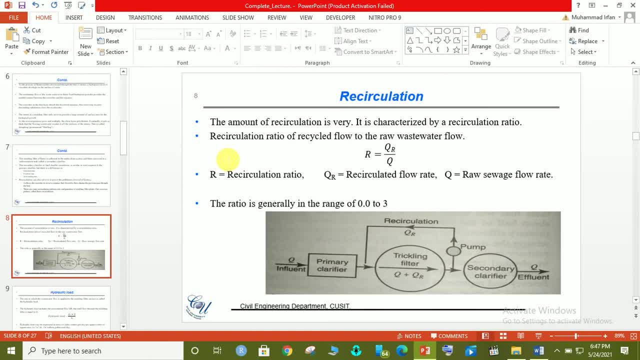 We call this as recirculation. The amount of recirculation is vary. It depends. It is characterized by a recirculation ratio. We define it as a ratio. It is a recirculation ratio of recycled flow to the raw waste flow. 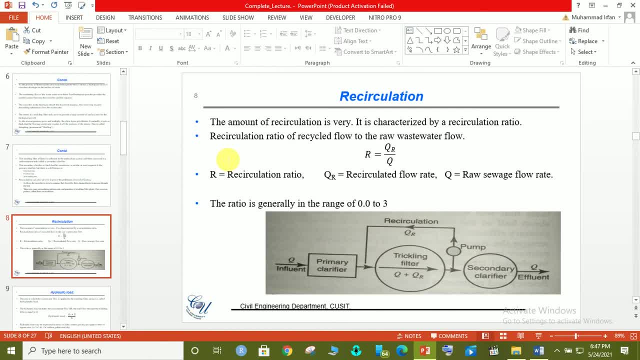 We recirculate it with a special ratio. We call R as recirculation, Q is R and Q is Q. We recirculate a particular portion of recirculated flow rate. Q is Q. We recirculate it. Q is R. 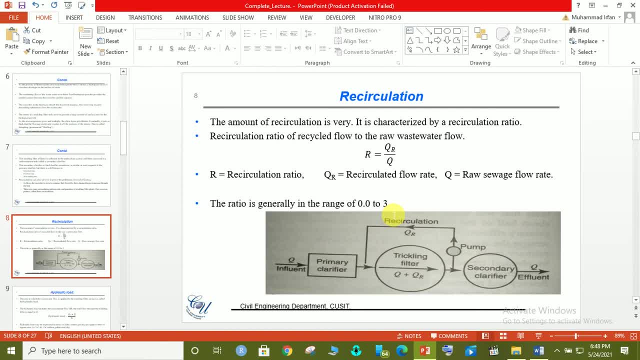 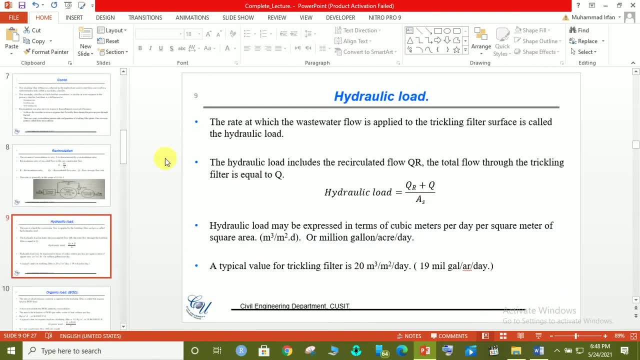 This ratio is between 0 and 3.. The second one is the hydraulic load. The rate at which the waste flow is applied to the trickling filter is called hydraulic load. The amount of waste water is from the primary effluent. The amount of waste water is applied to the trickling filter. 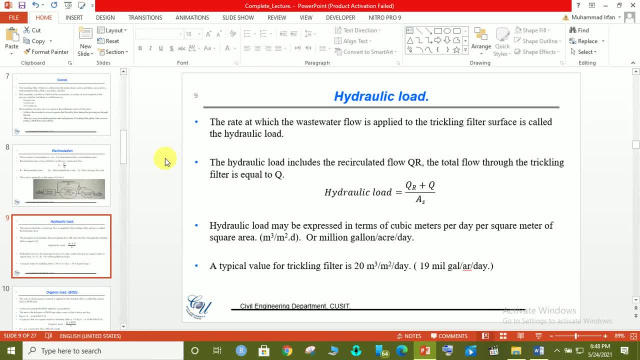 The amount of waste water is from the primary effluent. we apply the surface of the trickling filter on it and we call it hydraulic load. How much hydraulic load we apply on the trickling filter? So the hydraulic load includes the recirculated flow and the total flow through the trickling filter is equal to Q. 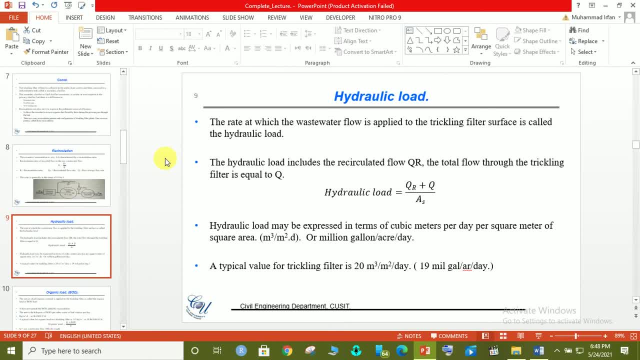 So the hydraulic load is equal to Qr plus Q. Q means the flow that comes from the primary and the recirculated flow is divided by the surface area of the trickling filter. This is called hydraulic load. So hydraulic load may be expressed in terms of cubic meter per day per square meter of surface area. 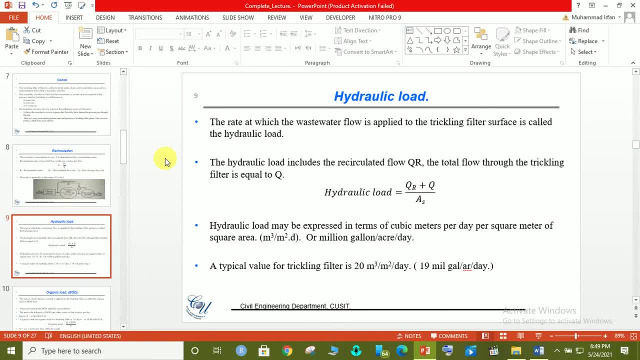 So cubic meter per day per square meter of square area. So we write it as M3 per M2 per day or Million Gallon per acre per day. It is the same thing. The value of hydraulic load for the trickling filter is 20 M3 per M2 per day. 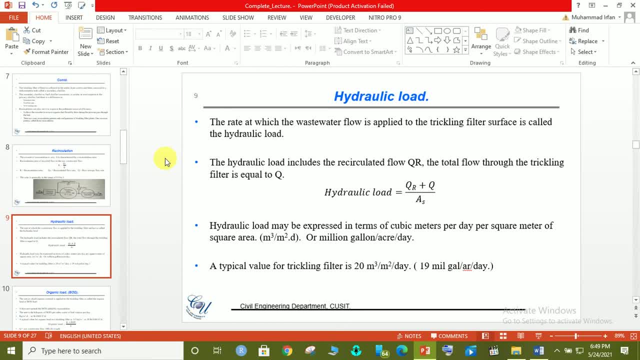 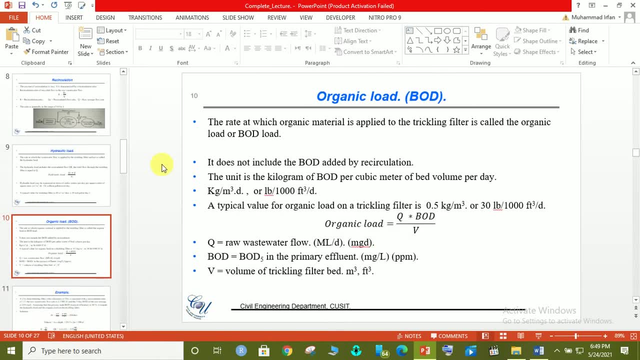 This is the typical value. It can be further or backwards. It is equal to 19 Million Gallon per acre per day. The other term is organic. look, just go get the beauty. the rate at which the organic material is applied to the trickling filter is called the organic load or beauty load. 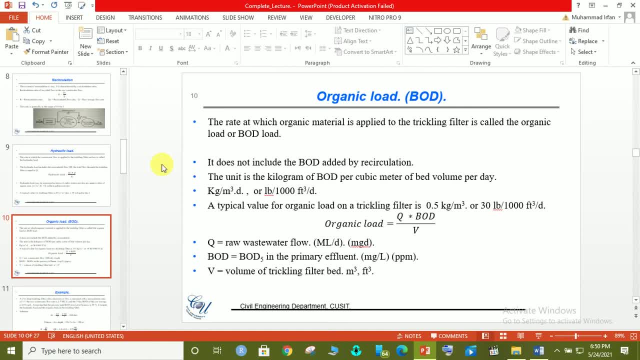 what's up, Joe? waste water home apply, collect a trickling filter pill. what's up, Joe? organic load? hey, just my organics hotel. just maybe you do at the head, Joe, rock hotel, bacteria, Kia, protozoa, key, it's gonna get the organic load. it does not include the beauty added by recirculation. looking this may. 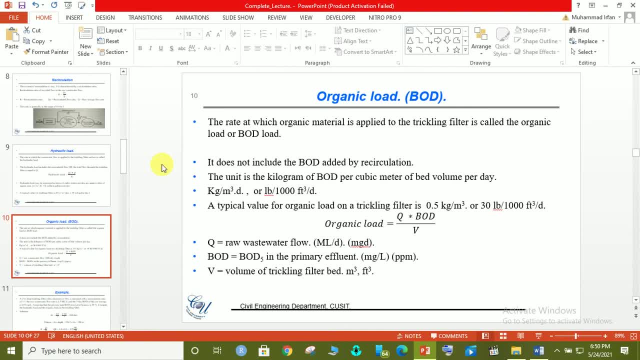 give me a man out Canada. okay, it's my woe beauty nahi hoti kinky. already hum take Martha by and incorporate. call it a to Jory circulation may beauty at the hand. well, I'm just make. only cut the unit and the is the kilogram of beauty. 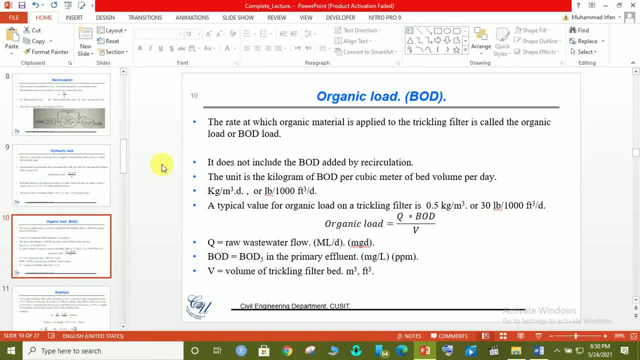 per cubic meter of bed volume per day, but the kg now a weight of beauty at the hair kidney. volume of water may per day. this guy, Joe, formula work. you multiplied by beauty, divided by volume, huge, have a raw waste water flow hand. but the primary influence I do at the a million liter per day may. yeah, 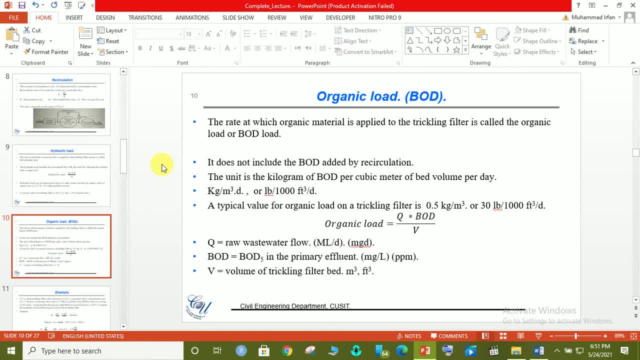 million gallon per day. may beauty 5 is the primary implement warm. let the beauty 5 beauty Q give you to beauty 20, you have ultimate hotel 20 kilo. I'm concerned eager sector. this damn beauty 5 you have all at the V is equal to. 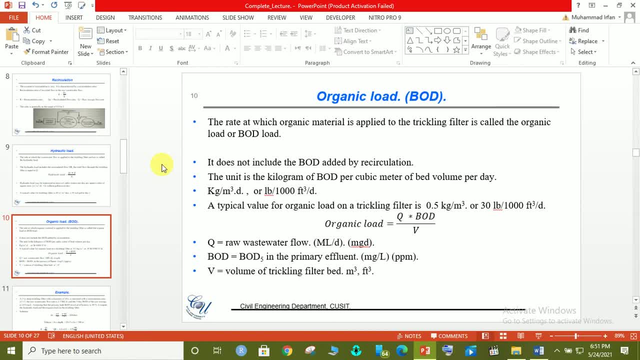 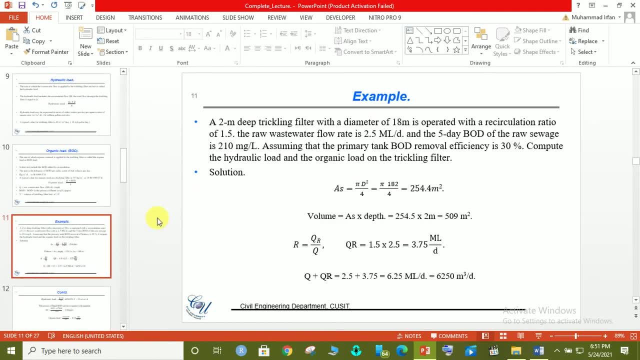 volume of the trickling filter. simple example: hand to me to do you trickling filter. I'm at a plastic trickle filter. had your two meter defy. with a diameter of 18 meters, operated with a recirculation ratio 1.5. the raw waste water flow rate is 2.5 million liter per day and a five-day beauty of the raw 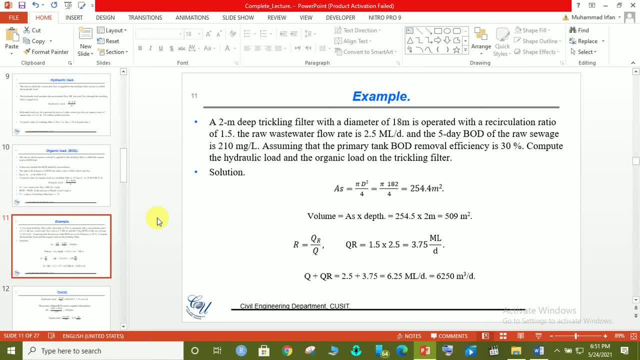 sewage is 210 million gallon per liter. yes, I did you say to have a given head to me, to deep hair depth, my repass, given a diameter, be given. have, Joe, recirculation ratio have. will be given a. are be given. have a look flow rate be given a Q is equal to will be given a five-day beauty. 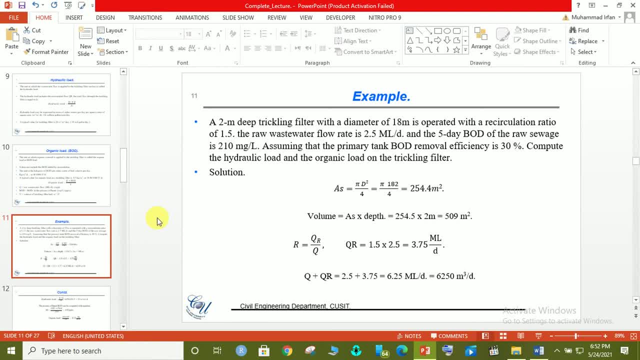 will be given, had 210 million gallon per liter and a milligram per liter. is you there? the primary change, that beauty removal efficiency is 30%- and I have a pause, Joe, primary tank, Joe, who thought I had my love, Joe, suppose about our capacity is water and 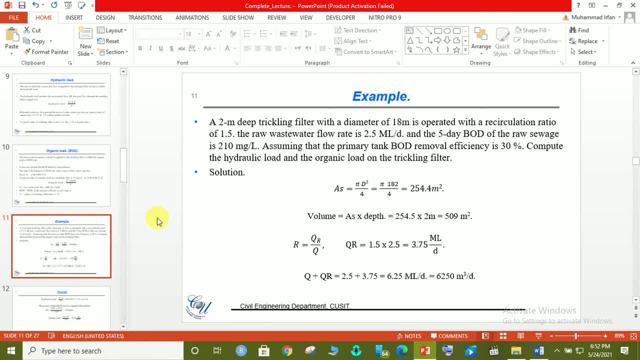 for up now swiss water go. primary treatment is reasonable primary treatment. suppose kiya to focus primary treatment. say beauty, do you have a 30 percent remove? okay, compute a mother, 70% a. be back here, Joe, just go home. they pass Karna a second treatment, say so, compute the hydraulic load and organic load on a. 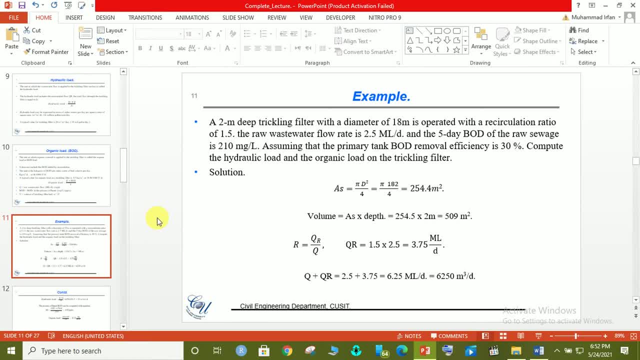 trickling filter. this capability, hydraulic load or organic loads have opened so surface area. I'm gonna pass a PI DSK divided by four per square metric second. we haveatz just five hundred five exercise tickets. that is 3 and a half fluid is on lump pad address. 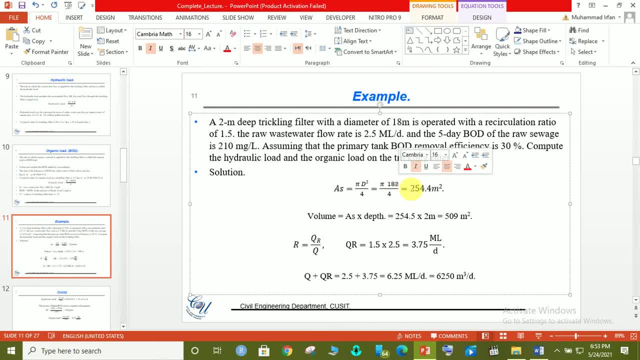 quick. I'm nothing multiple about lying over the table tutorial. have you all time? can you get back just a very strong meanwhile surface area of the way before that so we can know its volume from surface area multiplied by depth? so surface area is 254 and depth is 2. 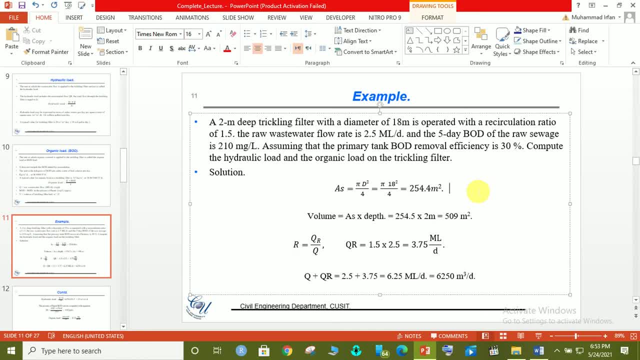 so it is 509 m2. so recirculation ratio is Qr divided by Q, so recirculation value is 1.5 given and raw waste Q is 2.5 mL per day. so we can know recirculation flow because we have Q given and R given. so we can know Qr easily. 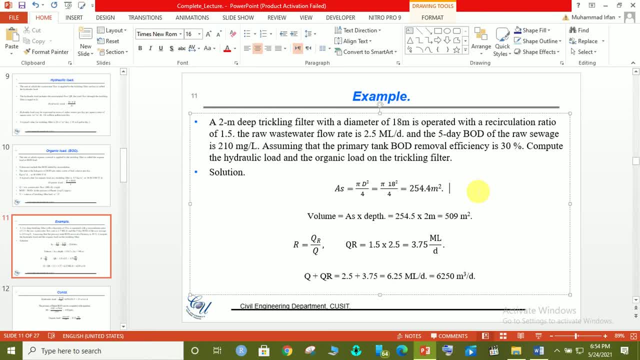 so it is 3.75 mL per day. so if we add Q and Qr, 2.5 plus 3.75, so it is 6.25 mL per day or 6.250 m3 per day. so this is called compute the hydraulic. 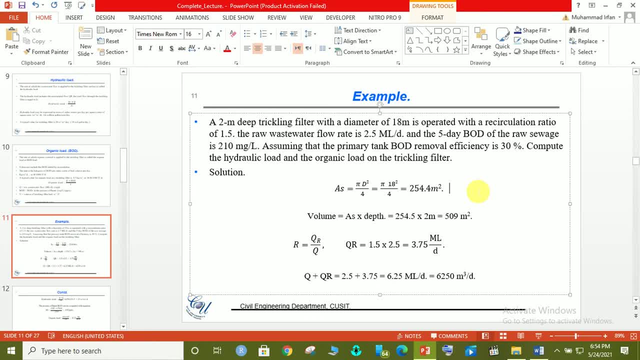 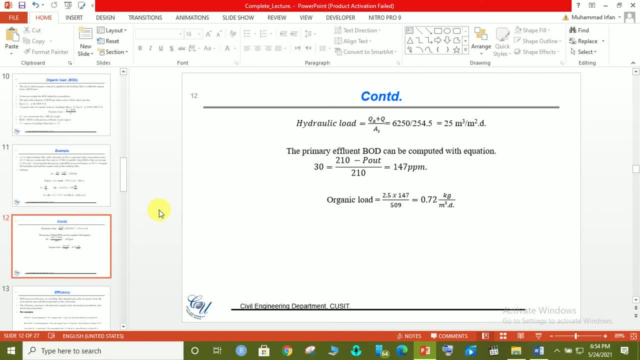 load and organic load on the trickling filter. so this is what we get. so hydraulic load is equal to Qr plus Q divided by S. so Qr plus Q is 6.250 m3 and surface area which we have calculated. so this is the hydraulic load. 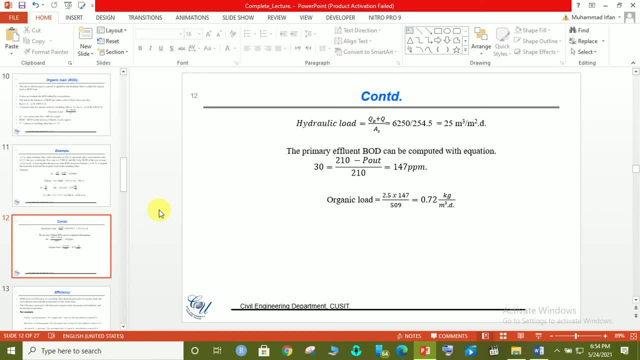 so the primary effluent, BOD, can be computed with equation. so this is the equation 30 is: the efficiency of primary effluent is equal to the BOD minus Poutput divided by the BOD input, which is the input, which is 1.47 part per million. 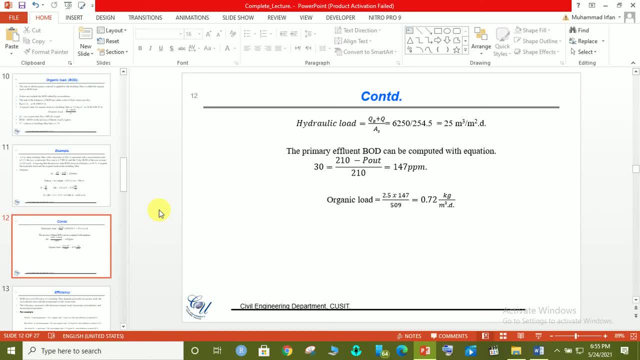 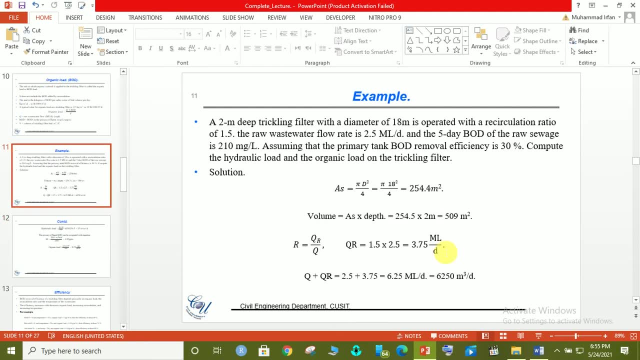 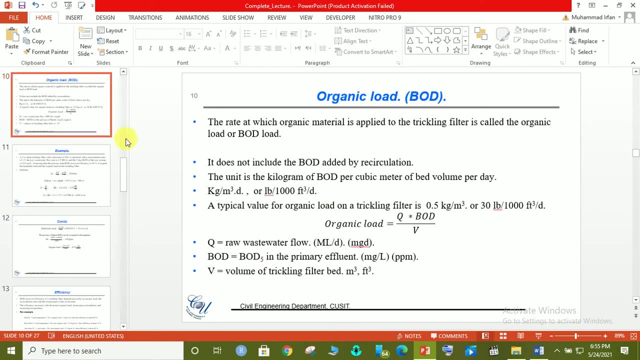 so with this we will know the organic load: 2.5 multiplied by 1.47, divided by 509, which we have known here the volume. so we will divide it by this volume. so we have organic load here, because the organic load formula is Q multiplied by BOD divided by V. 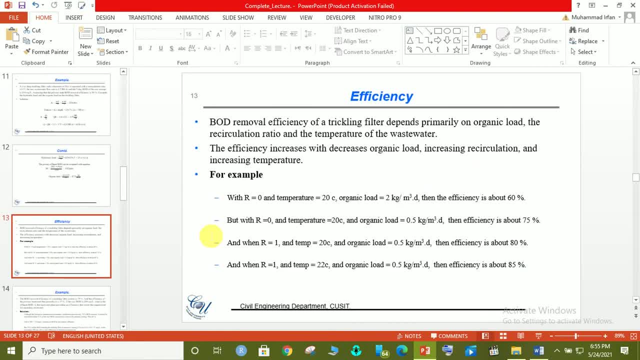 so this is what we have got: efficiency. so BOD removal efficiency of trickling filter depends primarily on organic load. the efficiency of BOD removal- suppose we have an extrinsic filter so we remove BOD from it. so it depends on primary load, organic load. suppose you have. 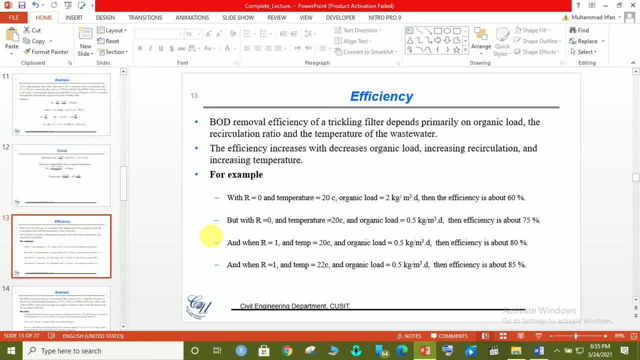 in any waste water, organic load is more so. this means that BOD removal will be more if its recirculation depends on ratio and temperature. if temperature is more, then BOD removal will be more. if it is less, then it will be less. the efficiency increases with decrease. 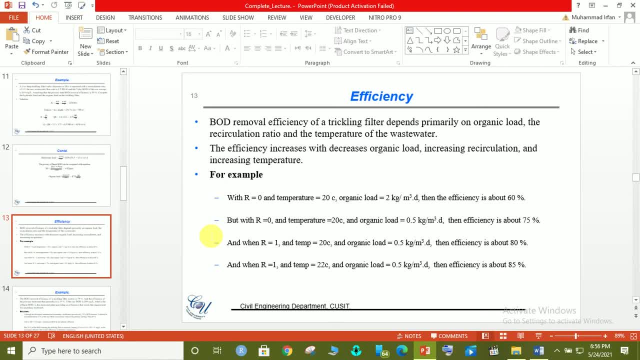 decreases organic load. suppose we have organic load which is more so. this means that the efficiency of any tank will be less. the efficiency increases with decrease organic load. in this way increases recirculation. if we want to increase efficiency, if we increase recirculation, then efficiency will be more. 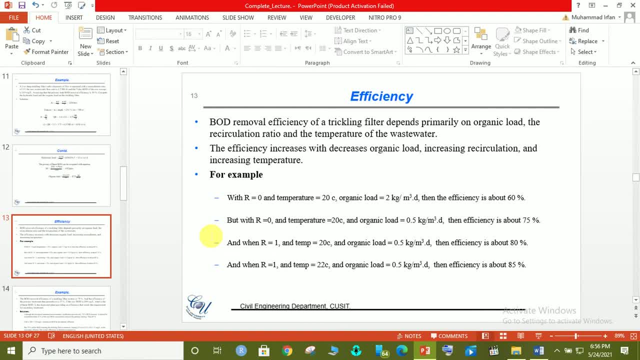 and if we increase temperature then efficiency will be more. these are some examples. suppose recirculation value is zero, temperature is 20 degree c, organic load is 2 kg per meter cube per day, so efficiency will be 60%. these are some facts. then same temperature is equal to 20 degree c. 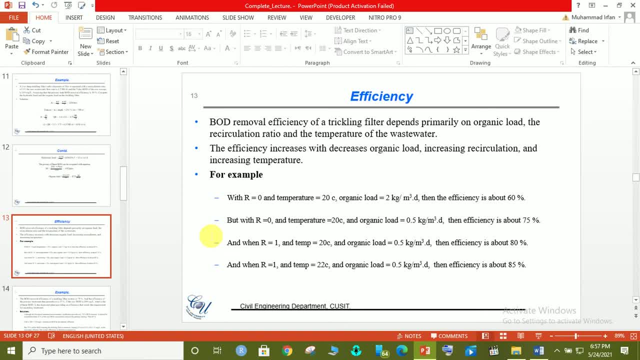 but we have reduced organic load here. we have reduced organic load to 0.5 means by decreasing organic load your efficiency will be increased. so if in the same scenario you have decreased organic load to 0.5, then your efficiency is 75%. but if you have increased recirculation, 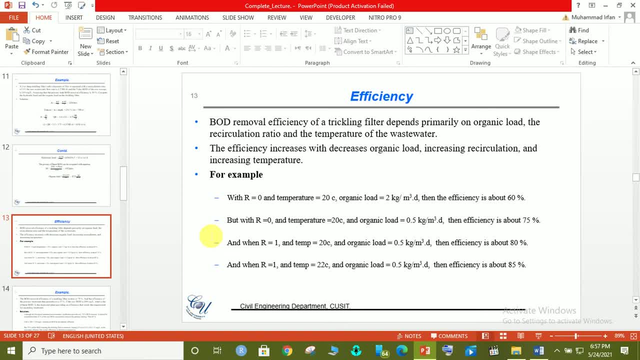 then your efficiency will be more. you can see that efficiency increases with increased recirculation. so if we have kept the same temperature- 20 degree c, organic load at 0.5 degree c- but we have increased recirculation, then your efficiency will be 80%. 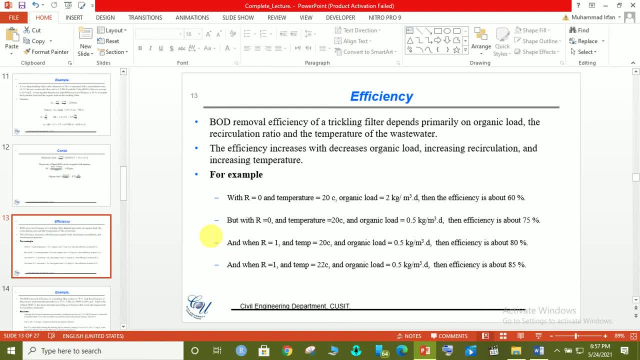 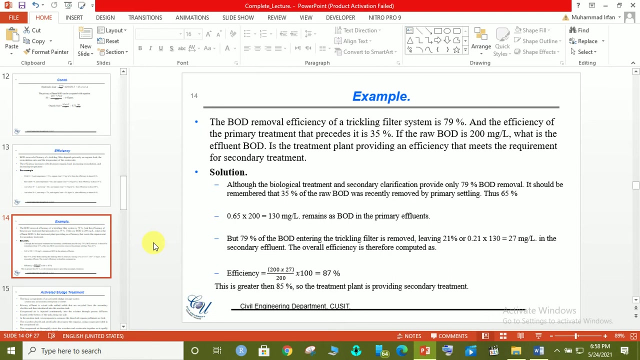 in this way: if recirculation is 1 but we have increased the temperature 22 degree c and organic load is 0.5, then your efficiency will be 85%. you can see that it depends on all three. this is another problem. the BOD removal efficiency of a trickling filter system is 79%. 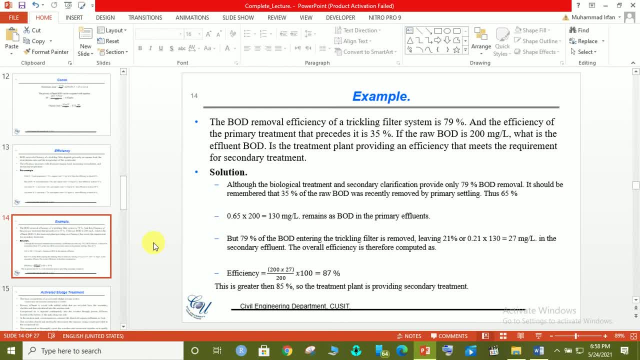 and the efficiency of the primary treatment that precedes it is 35%. you have to understand this a little. if the raw BOD is 200 mg per litre, what is the effluent BOD? is the treatment plant providing an efficiency that meets the requirement for the secondary treatment? 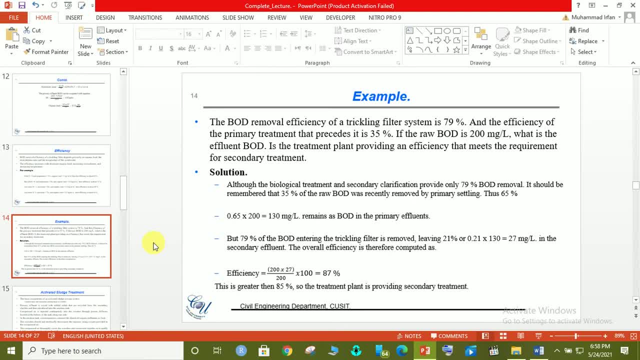 we have a trickling filter which efficiency is 79% and the efficiency of the primary treatment- the efficiency of the previous primary treatment- is 35% if the raw BOD is 200 mg per litre. if you have a BOD of 200 mg per litre, 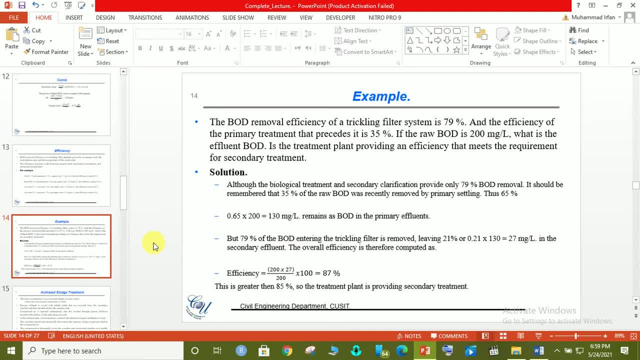 in any water. so what is the effluent BOD? what should be your effluent BOD means, if you have, what is the effluent BOD, what should be your effluent BOD? is the treatment plant providing an efficiency that meets the requirement for the secondary treatment. 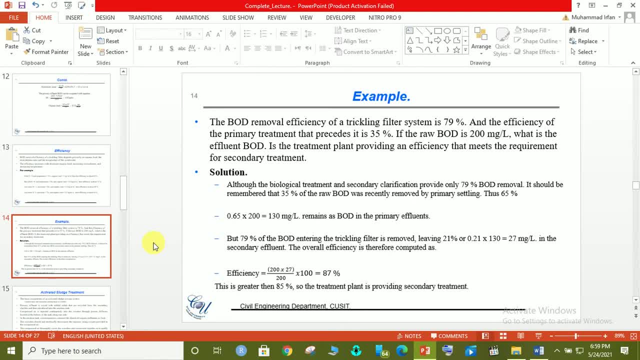 you have found the efficiency or does it meet the needs of the secondary treatment, although the biological treatment and the secondary clarification provide only 79% BOD removal? you can see this: the BOD removal is 79%. on the secondary treatment, the BOD removal is 79%. 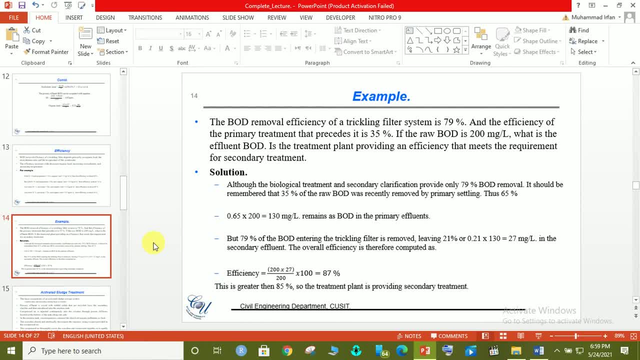 on the secondary treatment, it should be remembered that 35% of the BOD was recently removed by primary settling. so in this question that 35% BOD is the efficiency of the primary treatment means 35% removal is done there, so we have 65%. 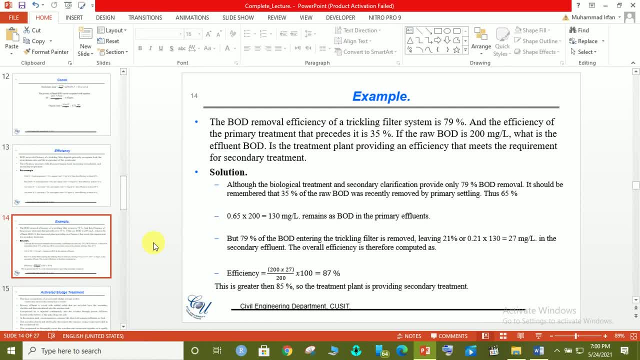 remaining 35%, 35%, 35%. the removal happened from the primary treatment. suppose if the BOD is given 200 mg per litre and we pass that BOD from the primary treatment, so its efficiency, which is given 35%, 35%. 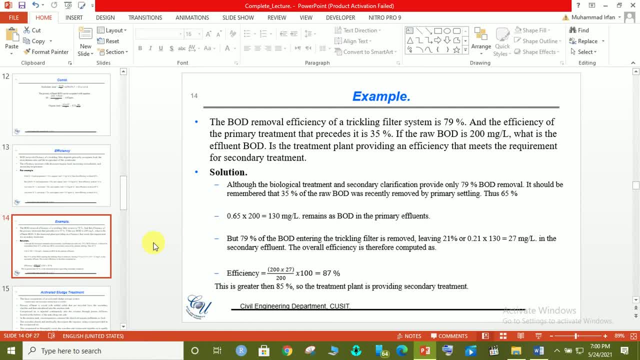 means the BOD, 200 mg per litre. 35% of that BOD is removed from that primary treatment. 35% is removed from that primary treatment. rest we have 65% BOD. so how we convert 65% in mg per litre, simple: we will multiply it. 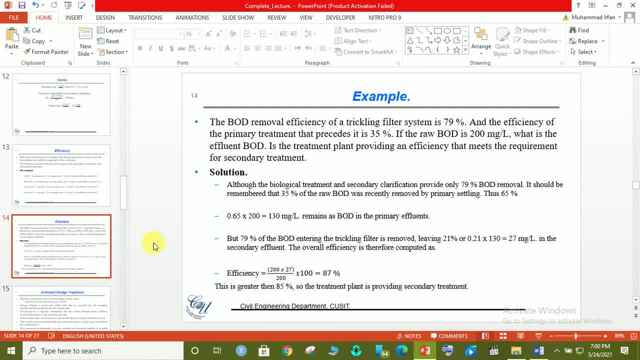 by total 0.65, it means that 130 mg per litre remains. if you want to know how much BOD is converted in undissolved form in the primary treatment, then you have to multiply it by 0.35. 0.35 multiplied by 200, because 35% BOD is converted in the primary treatment but the 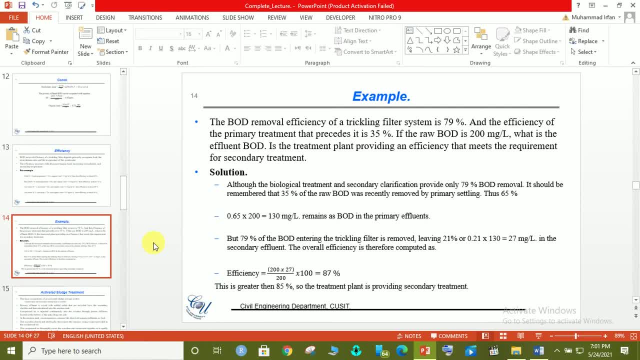 79% of BOD entering the trickling filter is removed, which is given in the question. 79% of BOD is of trickling filter, leaving 21%. if you see 79% of BOD is of trickling filter- not 100%, but 79%- means if you have total BOD of 200, then 79% of BOD will be removed. 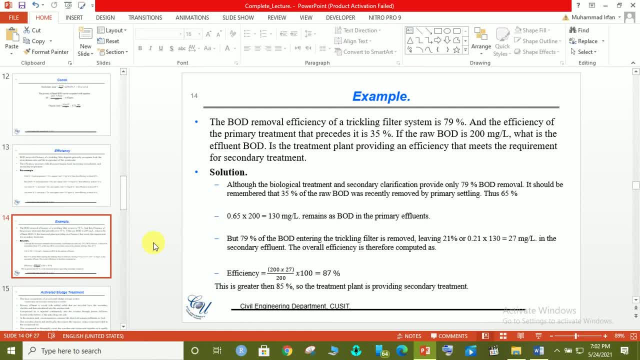 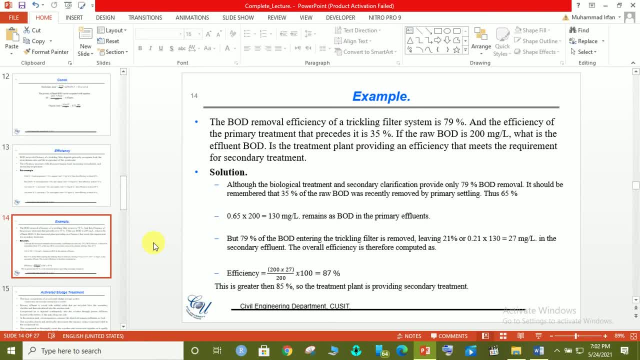 so the same primary treatment we passed with the trickling filter. then we passed the 130 mg BOD with the trickling filter. so now we will take only 130 mg, because the remaining 35% is already removed from the primary treatment. so we will simply multiply 130 mg by 0.21, which is 27 mg per litre. 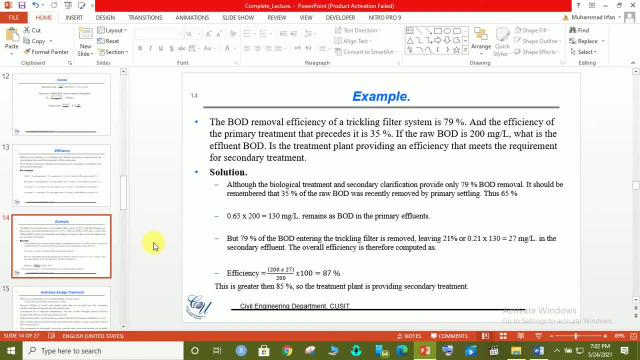 so this means if you have BOD of 200 mg per litre, which we passed from the primary treatment, then 35% of BOD is removed, which is 130 mg. so we passed the 130 mg BOD with the trickling filter, which is 130 mg BOD. 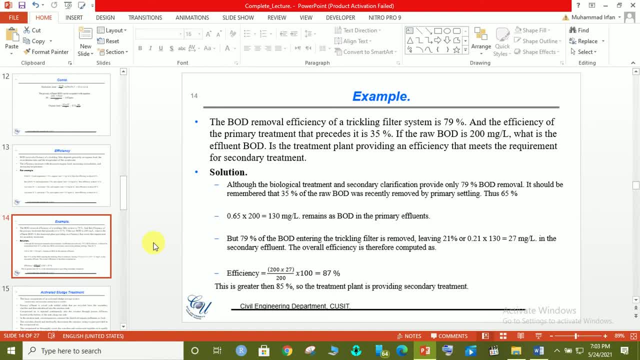 we passed the 130 mg BOD with the trickling filter, which is 27 mg per litre. so how will we know the efficiency of this? efficiency is equal to 200 multiplied by 27, divided by 200. this is the formula. so we have the total. 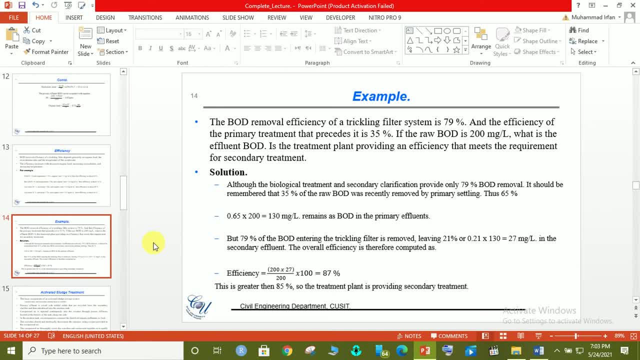 multiplied by the remaining, divided by the total, multiplied by 100, so this becomes 87%. so this is greater than 85%. so the treatment plant is providing secondary treatment. so for this, if it is more than 85%, so for this reason, we provide secondary treatment. 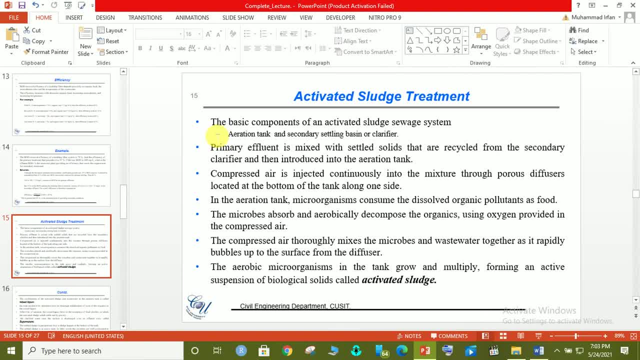 the next process is activated sludge treatment. the basic component of activated sludge sewage is aeration tank, secondary settling basin. and clarify there are two things: in this there is a tank and in that tank there is a aeration tank, in that we provide the air from below. 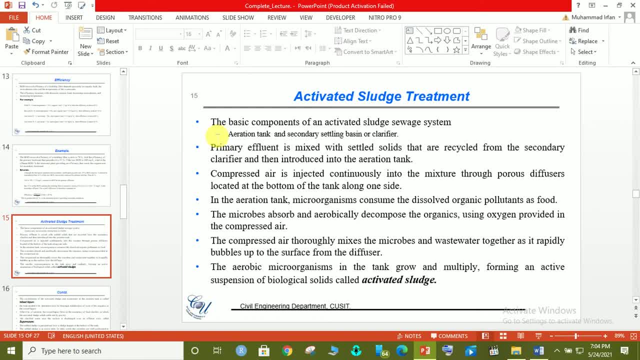 so that the particles remain suspended and the BOD, means the organics, remain suspended in that and the microorganisms in that remain suspended, and during that suspension it starts its metabolism reaction and in this way the process, the trickling filter is in the activated sludge. 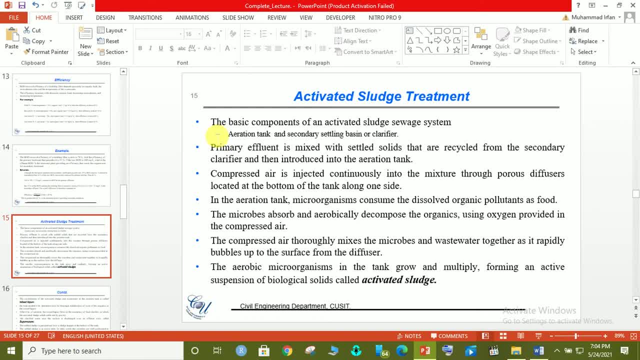 but there is a fixed filter and on that microorganisms are attached and the wastewater we pass through that filter. but in activated sludge there is a suspended system. the compressed air is injected continuously into the mixture through the porous diffuser located at the bottom of the tank. 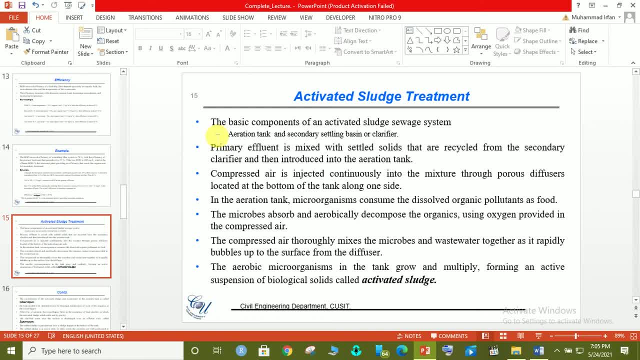 along one side. in this way we pass the compressed air so that the organics remain suspended in the aeration tank. microorganism consumes the dissolved organic pollutants as food. the same process of trickling filter. if we have microorganisms in that aeration tank, our food. 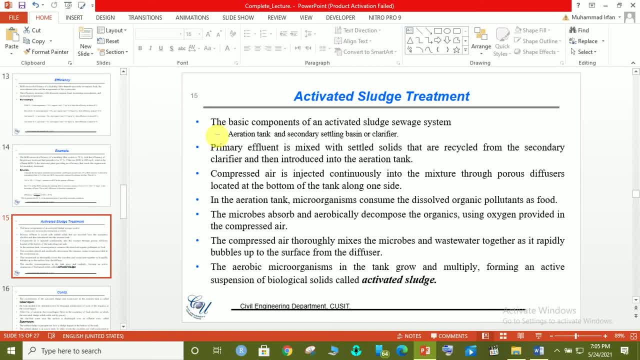 is taken from the dissolved pollutants in that wastewater. the compressed air thoroughly mix the microbes and waste water together as it rapidly bubbles off to the surface from the diffuser. the aerobic microorganism in the tank grow and multiply in this way if it continuously gets oxygen. 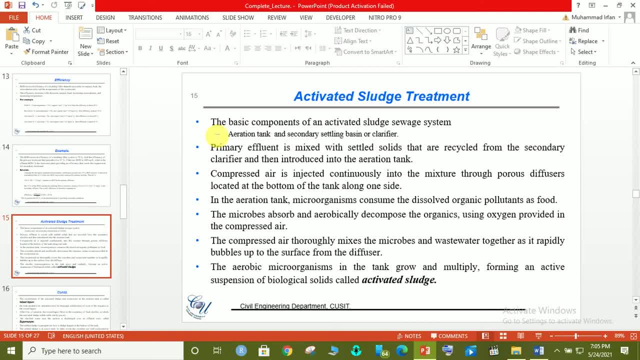 then this causes increase in the number of microorganisms in the tank. this is why we call it active suspension of biological solids or activated sludge, because this is always active. through the aeration process we provide the air, we provide the dissolved oxygen, so that all the microorganisms 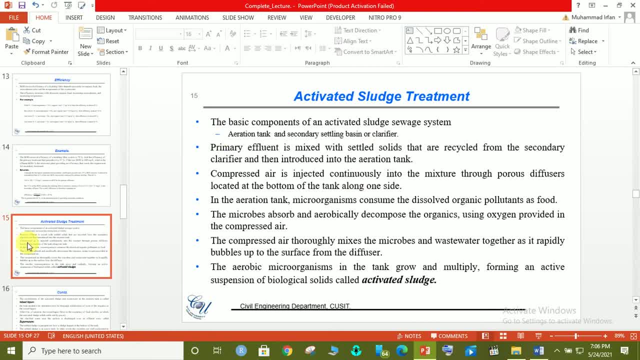 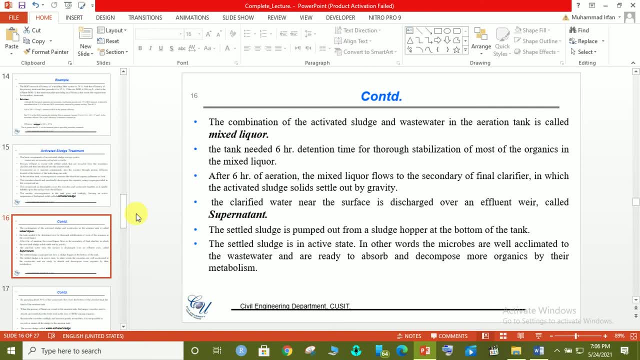 can multiply and increase in quantity. the combination of the activated sludge and the waste water in the aeration tank is called mixed liquor. there is no need in this. the retention time of this is 6 hours, which means that waste water after 6 hours when the bacteria 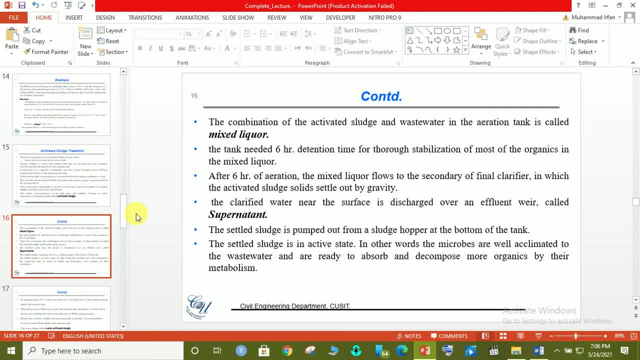 collect the waste water, the surface, the soft water that we collect that surface. we call it supernatant. the settled sludge is pumped out from the sludge at the bottom of the tank. the shape of the sludge is at the bottom and in that the solids remain. 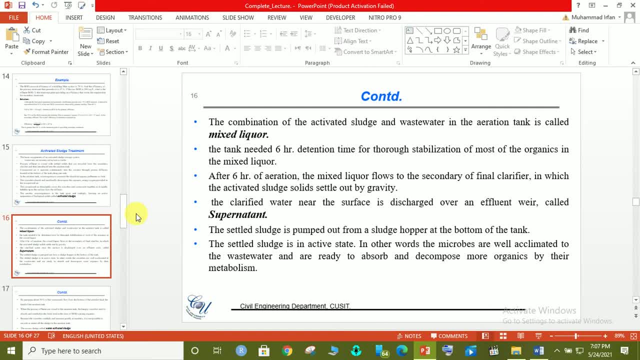 the sludge is an active state, in other words, the microbes are well accumulated to the waste water and are ready to absorb and decompose more organics by their metabolism. the sludge that sits at the bottom still has the same power, so that the dissolved particles 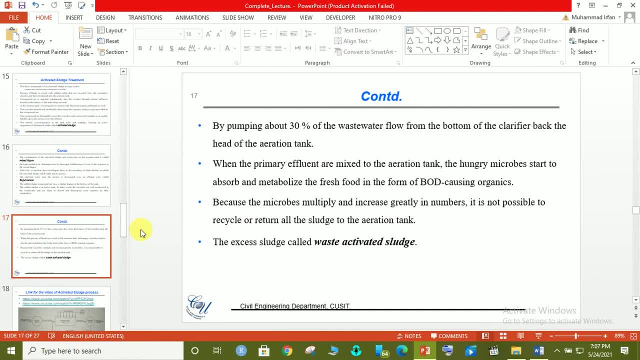 can be absorbed and converted into undissolved form. by pumping about 30% of the water flow from the bottom of the clarifier back to the head of the aeration tank. the recirculation process is done here because in the sludge the bacteria or microbes 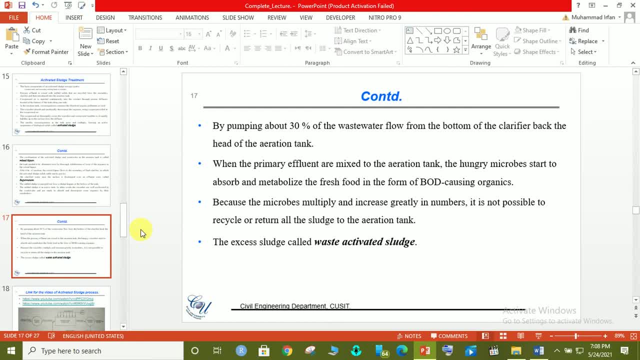 are active. that is why, when we take 30% of the waste water back to the aeration tank so that the active microbes can absorb the dissolved particles from the waste water, when the pumping effluents are mixed to the aeration tank, the hungry microbes start to absorb. 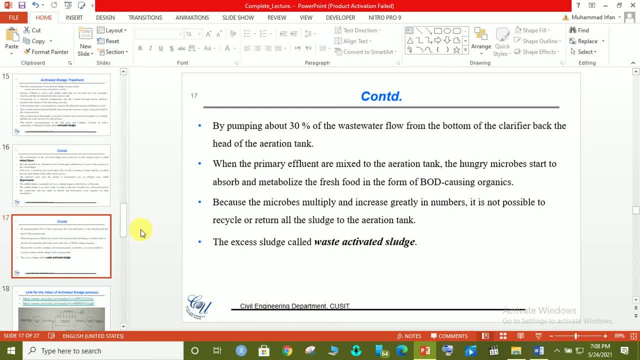 and metabolize the fresh food in the form of beauty, causing organics, because the microbes multiply and increase greatly in number. it is not possible to recycle or return all the sludge to the aeration tank. because of this, we do not recycle all the waste water. 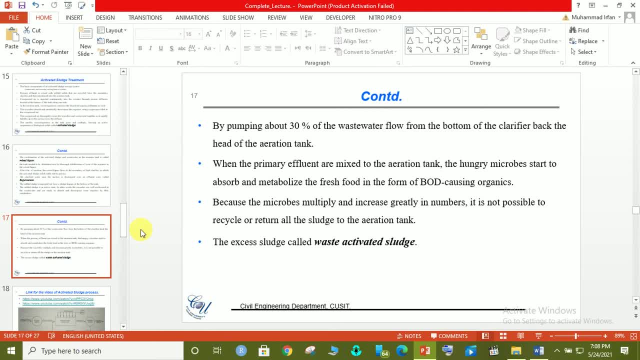 like we recycle in the trickling filter. we do not recycle 30% of the waste water here and take the rest to the next process, the excess sludge, called waste activated sludge. the excess sludge is called waste activated sludge. you can see we have sewage effluent. 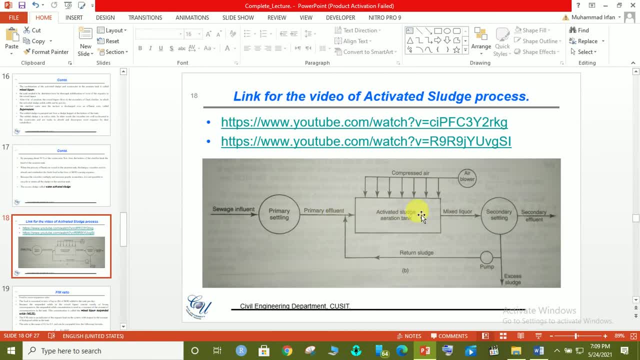 which comes to the primary settling tank. from there activated sludge. there was a trickling filter. here is the activated aeration tank. we pass this process and bring it to the secondary settling tank. we pass it again. you can see, we take the waste. we take the waste. 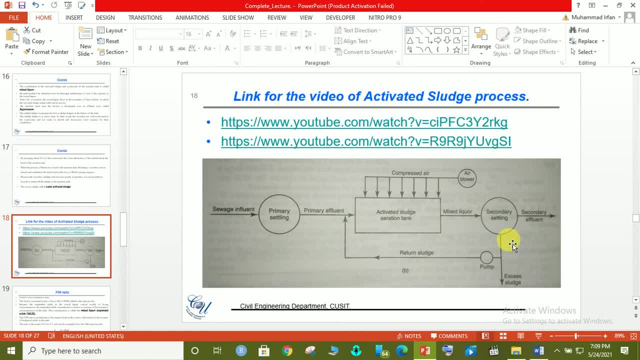 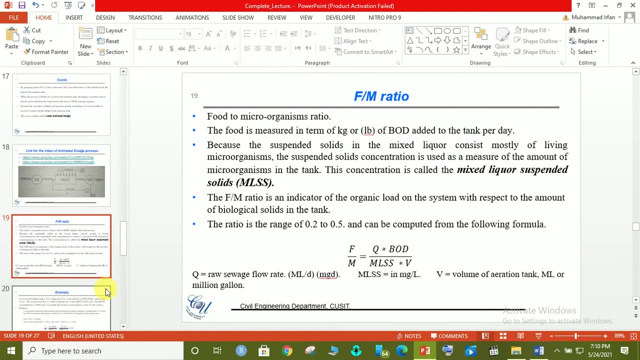 again because the microbes are in active state. we take it again so that the dissolved particles, the active microbes can diffuse the dissolved particles. there is a ratio, we call it fm ratio, food to microorganism ratio. so the food is BOD, the food of microorganism. 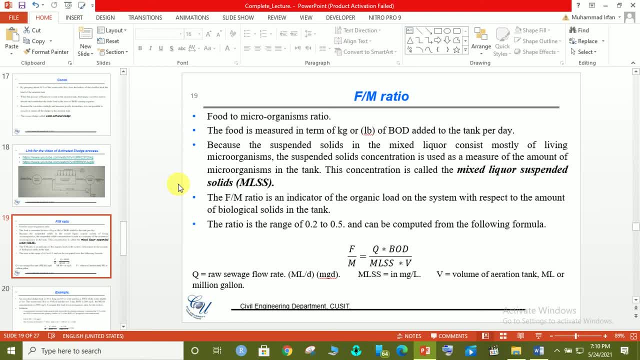 is BOD dissolved or suspended organics, because the suspended solids in the mixed liquids consist mostly of living organisms. the suspended solids concentration is used as a measure of the total microbes in the tank. this is called mixed liquids suspended solids. its range is from 0.2 to 0.5. 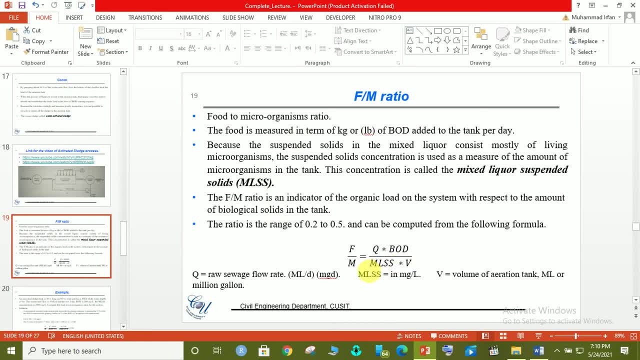 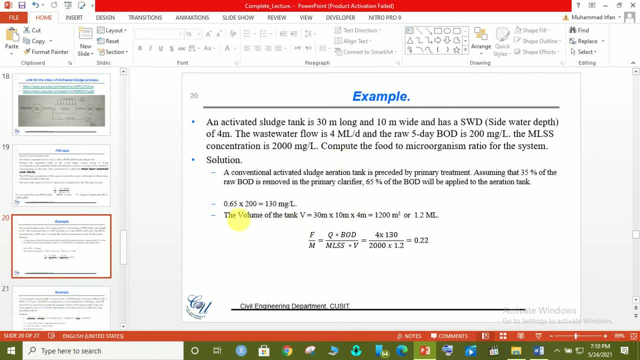 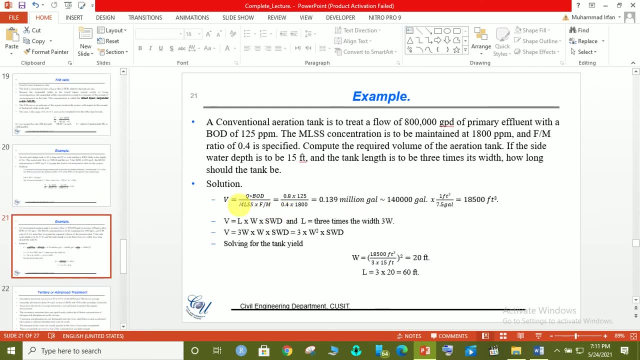 the formula is: Q multiplied by BOD. mixed liquids- suspended solids multiplied by volume. there is an example. you can see. it is an easy example. everything is given. you just have to put it in. this is an example. you just have to put it in. there is nothing else. 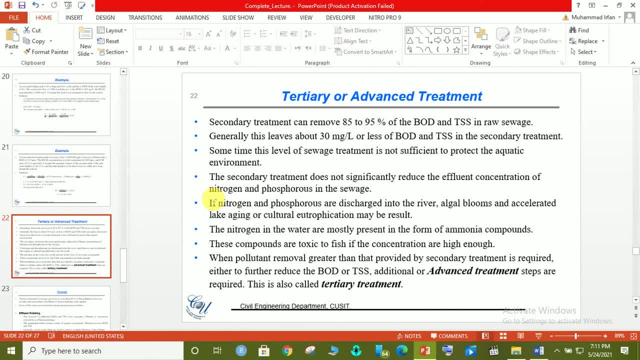 the next one is the tertiary or advanced treatment. when you pass the water from the secondary treatment, 85-90% of your beauty total suspended solids is removed, but still your 5% or almost 10-15% is left. generally this leaves about 30 mg per litre. 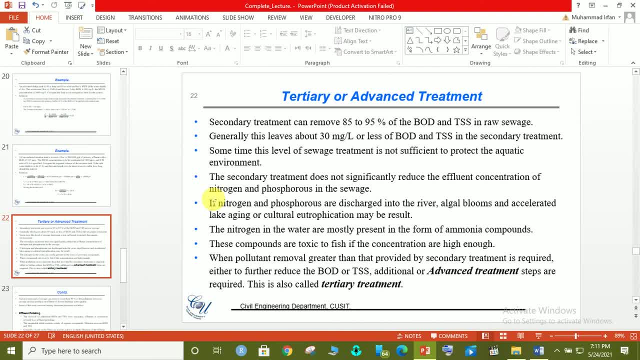 or less of beauty and total suspended solids in the secondary treatment. so sometimes this level of sewage treatment is not sufficient to protect the aquatic environment. suppose 30 mg per litre is still left, then you have to pass it from the tertiary or advanced treatment so the secondary treatment. 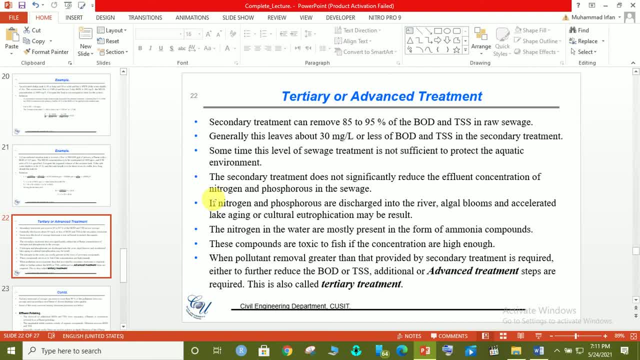 does not significantly reduce the effluent concentration of nitrogen and phosphorus in the seawater. if you have nitrogen or phosphorus compounds present in the water then they do not pass through the secondary treatment. you have to pass it from the tertiary or advanced treatment so that the nitrogen 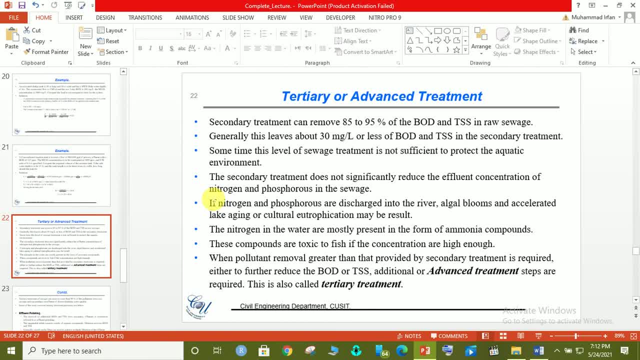 is removed or the phosphorus is removed, if the nitrogen and phosphorus are discharged into the river. if you have not done tertiary treatment, and nitrogen and phosphorus are present in the same water, and if you have discharged it in any river, then the algae in the green colour 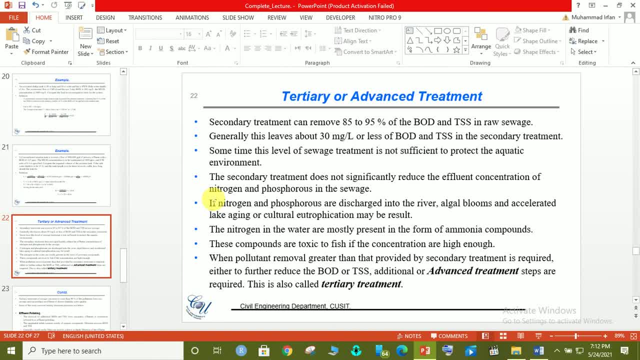 will be accelerated more in that water. after some time it will start to form, so the nitrogen in the water are mostly present in the form of ammonia compound. this is obvious because we use ammonia and phosphate for agriculture. these compounds are toxic to fish if the concentration is high enough. 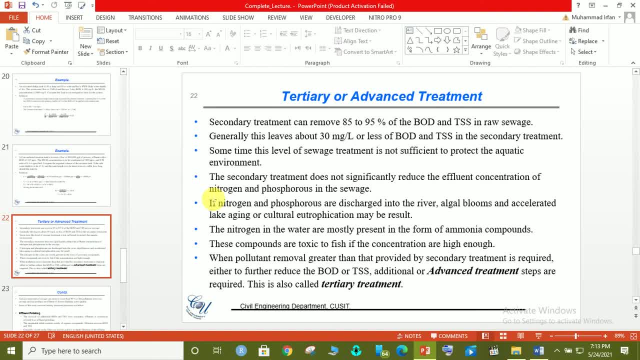 when pollutant removal, the secondary treatment is required. either to further reduce the BOD or TSS, additional or advanced treatment are required. this is called the tertiary treatment. if you have to decrease the BOD or TSS level, then you have to pass it through tertiary treatment. tertiary treatment remove almost 99% of the pollutants from the raw sewage. some of the most common tertiary treatment process. the first one is effluent polishing. what does this mean? the removal of additional BOD and TSS from the secondary effluent is sometimes referred to. 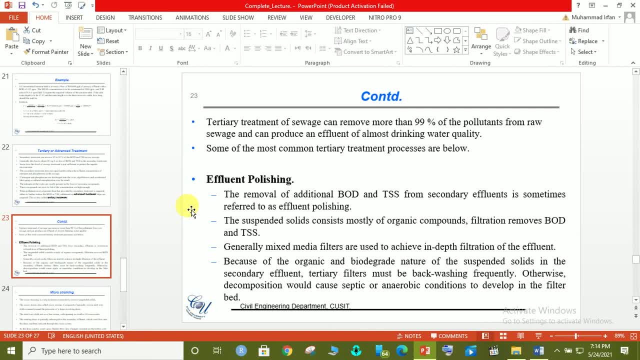 as effluent polishing. the BOD or total suspended solid that comes from the secondary is called effluent polishing. the suspended solid consists mostly of organic compounds. filtration removes BOD and TSS. generally, mixed media filter is used to achieve in depth filtration of the effluent. 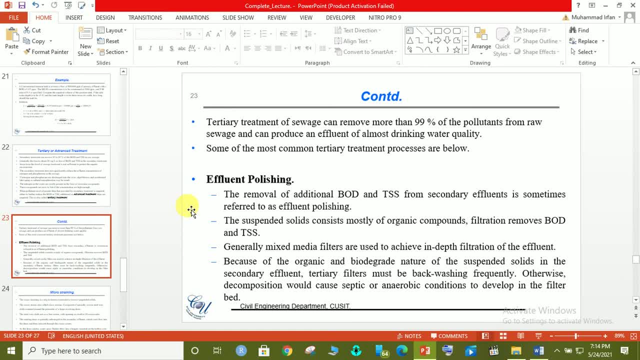 because of the organics and biodegrade nature of the suspended solid and the secondary effluent, tertiary filters must be back washing frequently. this is the same procedure. the effluent polishing is done in this, the suspended solid or BOD that comes from the secondary effluent. 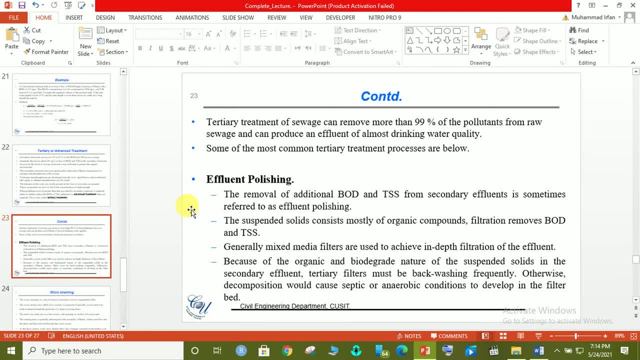 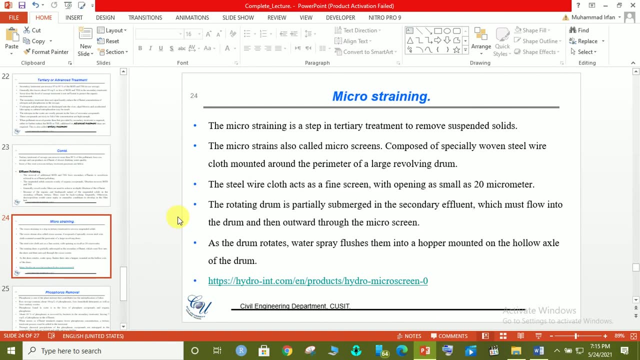 is filtered through mixed filter media. we pass it through a special depth filter so that the BOD and TSS can be removed. one is microstraining. the microstraining is a stiff and tertiary treatment, the microstrain, also called microscreen. this is also called microscreen. 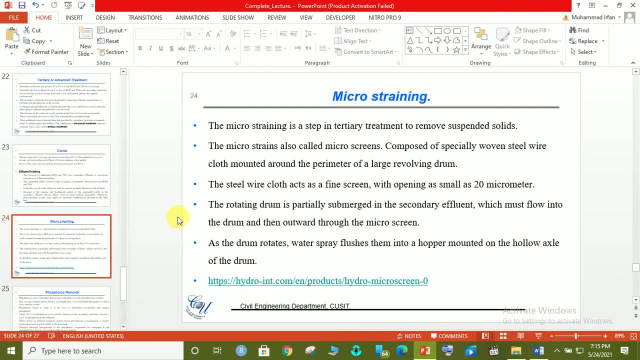 this is a drum shape composed of spherical steel wire cloth mounted around the perimeter of large revolving drum. we have a large revolving drum. on this drum there is a mesh and on that mesh there is a cloth. we pass that water through that mesh, or water and whatever is left on it. 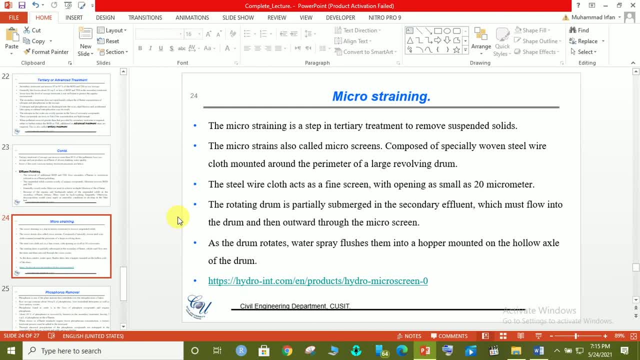 we flush it. the steel wire cloth with opening of as small as 20 micrometer rotating drum is partially submerged in the secondary effluent which must flow into the drum and then outward through the microscreen. I have given the link of this. you can see it. 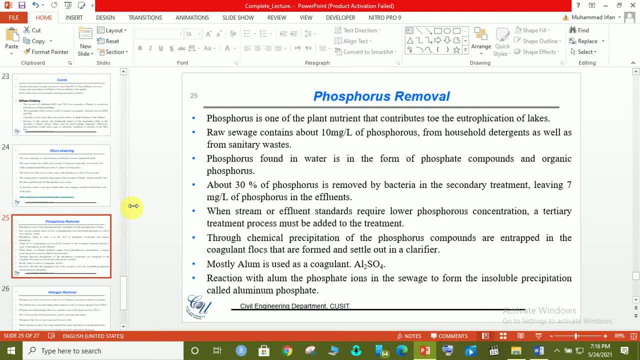 in the video. the next one is the pasporous removal. this also removes the pasporous. how do we remove the pasporous? to remove the pasporous, we do a chemical precipitation process. chemical precipitation means that the pasporous, which is in dissolved form, 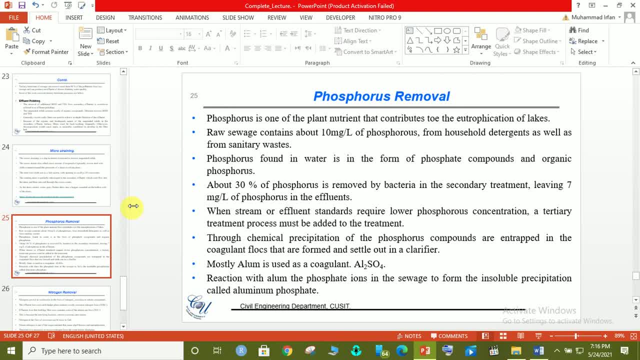 we have to bring it in undissolved form. to bring it in undissolved form we have to add some chemical. we call it coagulant. when you add that chemical it converts the dissolved particle in some other chemical compound in undissolved form. mostly we use alum. 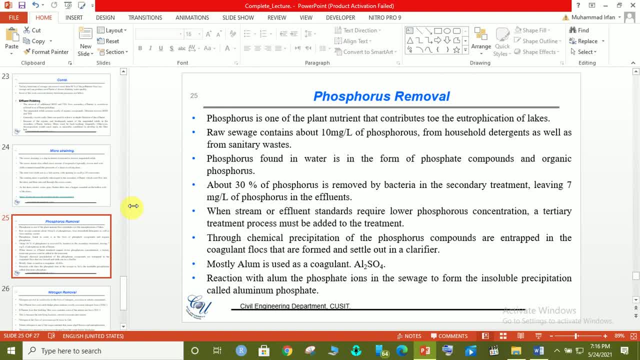 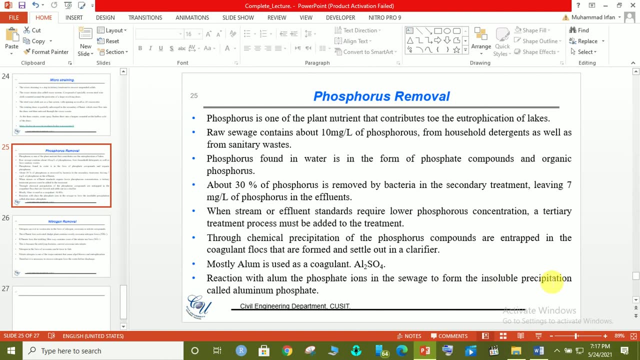 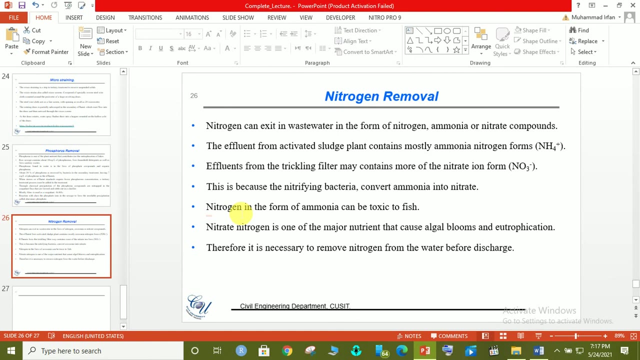 coagulant, which formula is AL2SO4- aluminium sulfate. when aluminium sulfate reacts with pasporate, it becomes your aluminium pasporate. aluminium pasporate sits down in insoluble form and we remove it. we also remove the nitrogen, because nitrogen is present in the form of ammonia.